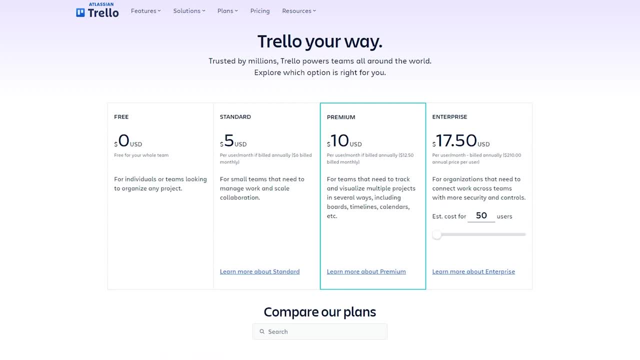 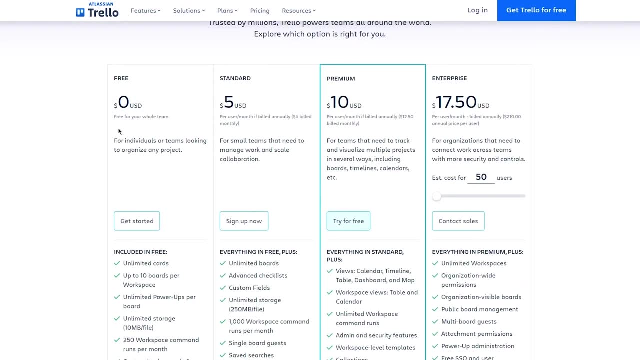 into it, you know. So first of all let's go ahead and discuss the pricings and plans for Trello. Now the four different pricings and plans are: first of all, there's the free plan. okay, Now in the free plan, obviously the money- zero dollars for individuals or teams looking to 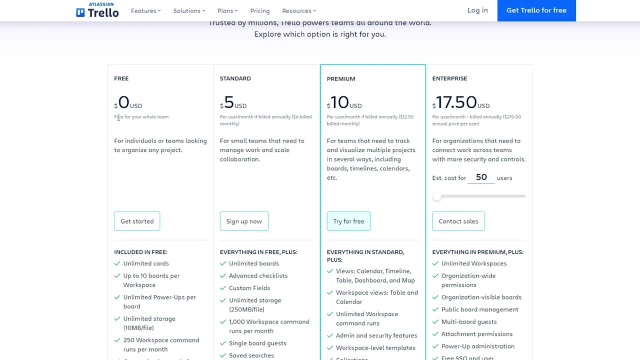 organize any project okay, And it's free for the whole team. Obviously, this is the fun thing and the good thing about Trello: like there's no trial or anything, It's like a proper full-fledged free plan and in this free plan, as you can see, you get pretty, pretty good features, like you know. 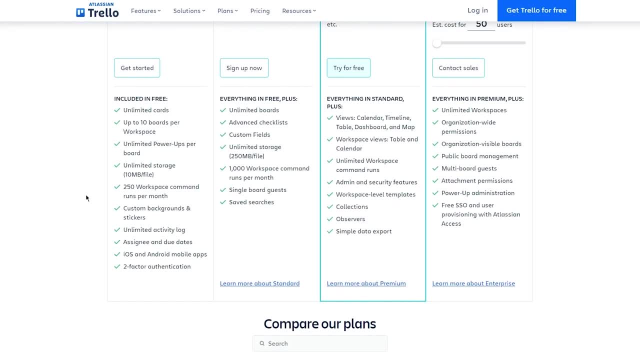 for unlimited cards. okay, Cards are basically, you know, the topics that you add in your board. Now unlimited cards, then you have up to 10 boards per workspace, Unlimited power-ups per board. You have unlimited storage, with which like 10 megabytes per file. 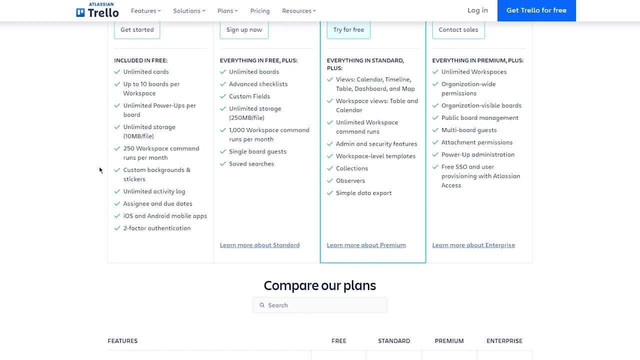 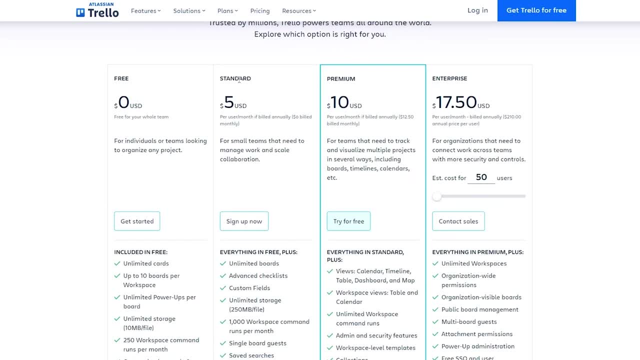 know much more features. then obviously you have the standard plan, which is obviously um the more you know- basic plan, which goes a bit above the free plan for small teams that need to manage, work and scale their collaborations. now this is, you know, five dollars and um it basically has. 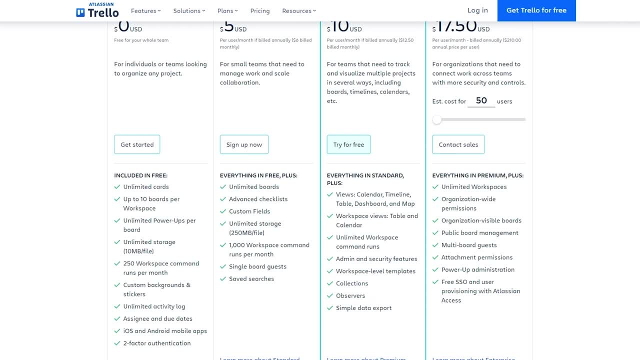 unlimited boards. in it you can choose to create as many boards as you can. as you can see, in free you can make up to 10. only so unlimited boards can be done in standard with you know the advanced checklists: custom fields, unlimited storage with 250 megabytes per file, 1000 workspace command runs. 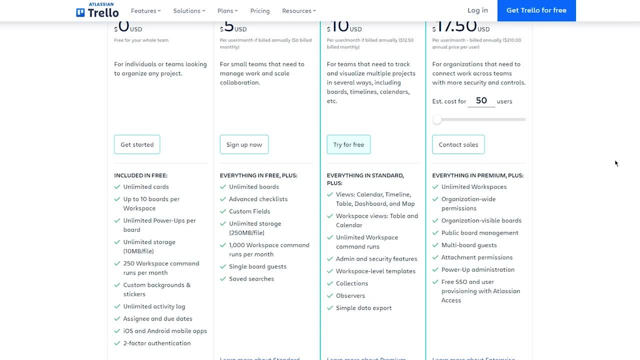 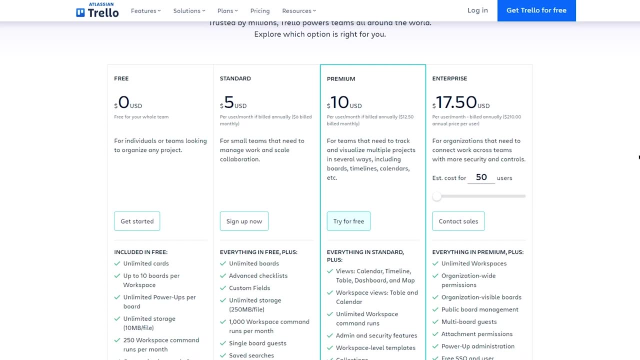 per month, single board guests and saved searches. then there's the most popular one, which is like the most used uh, which is the premium version, which is ten dollars, and it's for teams that need to track and visualize multiple projects in several ways, including boards, timelines, calendars. 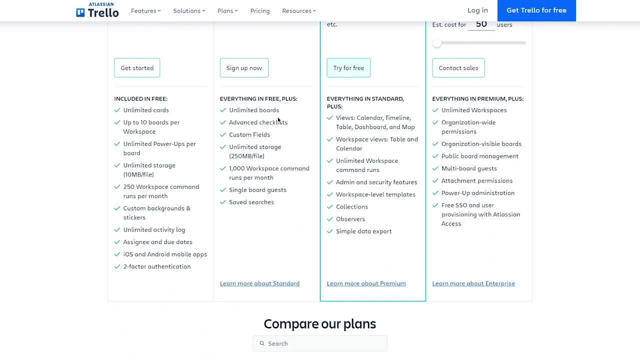 etc. and obviously the same features with, like you know, in the standard uh, plus this stuff, like all the different views, like calendar, timeline, table, dashboard and map, you have workspace views, table and calendar. unlimited workspace command runs admin and security features, collection observers. you know all that stuff. and then obviously comes enterprise. this is obviously for, like the big 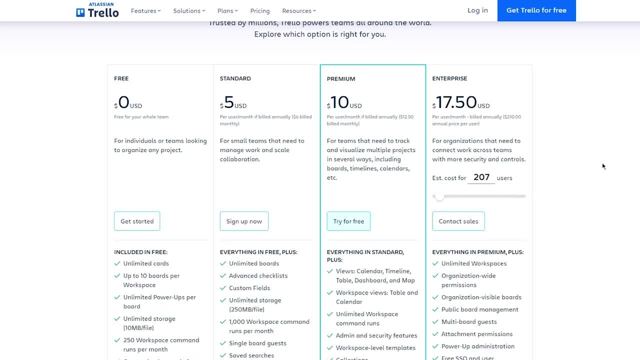 companies and i'm gonna stay out of this for now. but if you're like in a large-scale company and you wanna, you can just set up, you know, advanced folks that can manage them a little bit night and night put, like the few that probably are kind of designed forекст, so you can be a little bit more. 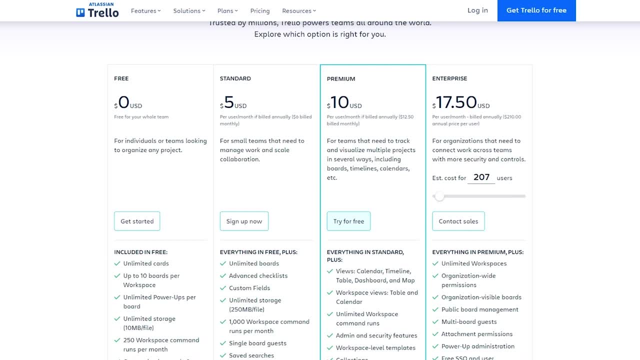 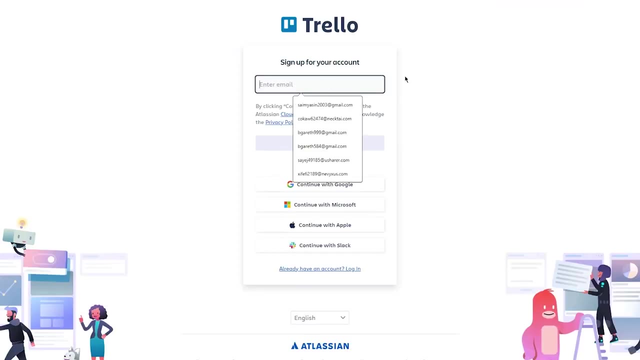 go ahead with this. you can. okay, that totally depends on you. but yeah, now if uh, like i were to, you know, get straight into the whole signup process, uh, for that, what i'm gonna do is i'm gonna go ahead and click on, get started over here, and once i do that, here it says sign up for an. 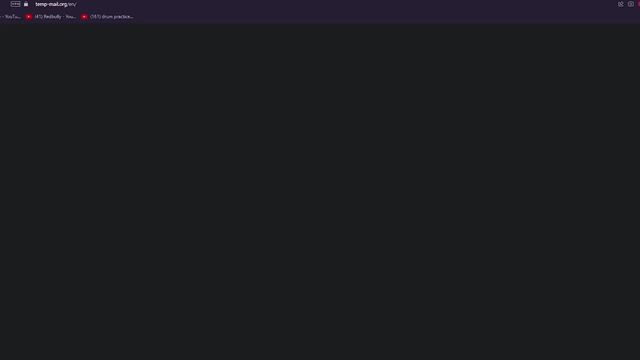 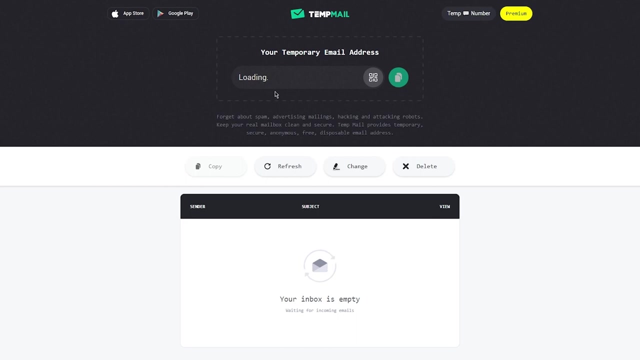 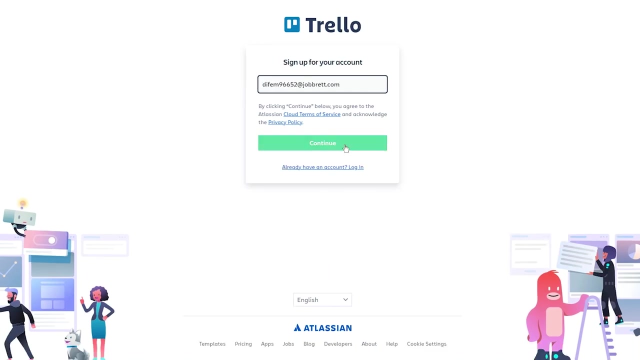 account. okay, now i'm gonna be using a temp mail. okay, a temp mail is a temporary email and i'm gonna be using that to sign myself up with trello. so let me just wait for my temp mail to load up and i'm gonna copy it and i'm gonna paste it here. now i'm using a temp mail, obviously. 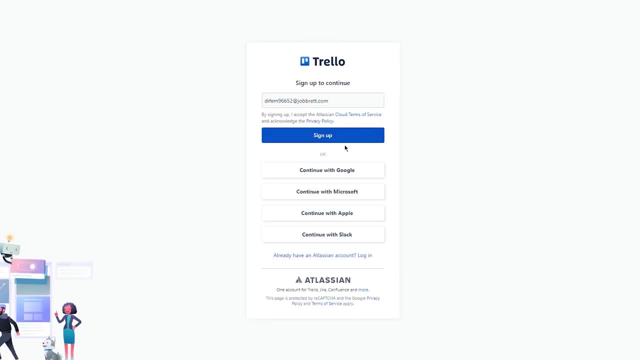 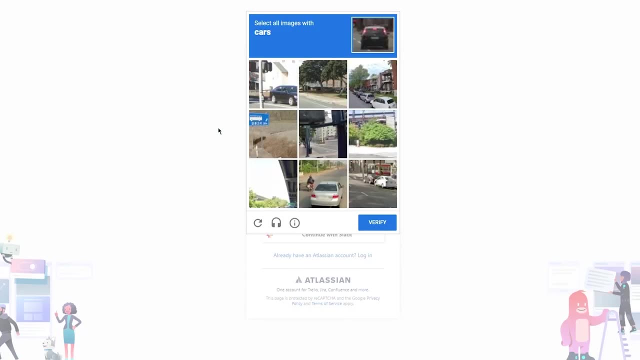 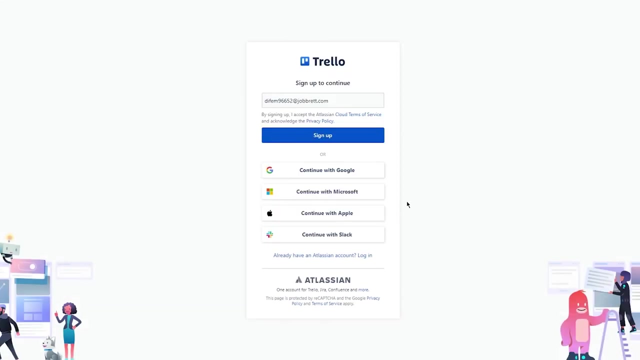 just because, uh, for like the video purposes, and once i use the temp mail, from there on out, what i'm gonna do is obviously dispose it after this video. so it all depends on you whether you want to use a temp mail or not. you can just use your, you know. 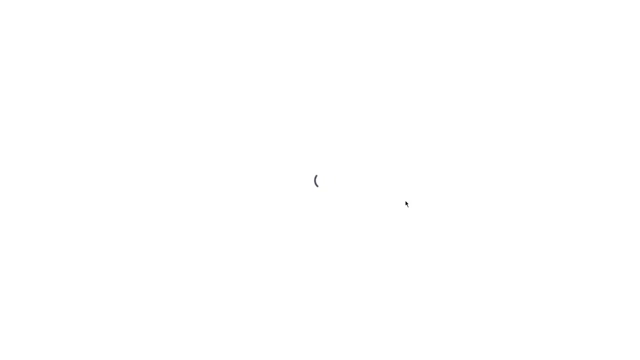 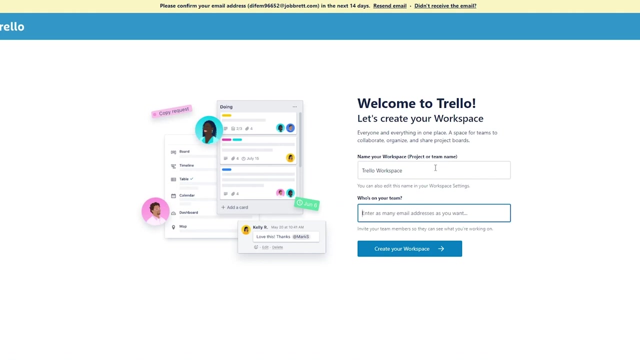 you can just use your, you know. you can just use your you know main google, gmail, uh, hotmail, yahoo, all that stuff, because that's just much you can say easier to use. now you're gonna head over here. welcome to trello, let's create your workspace. okay, now everyone. and 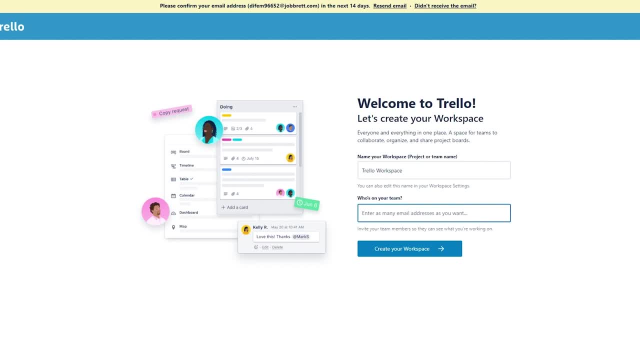 everything in one place: a space for teams to collaborate, organize and share project boards. name your workspace, project or team name. now you could obviously name yourself anything. i'm gonna name myself that. who's on your team. enter as many email addresses as you want. i'm gonna keep. 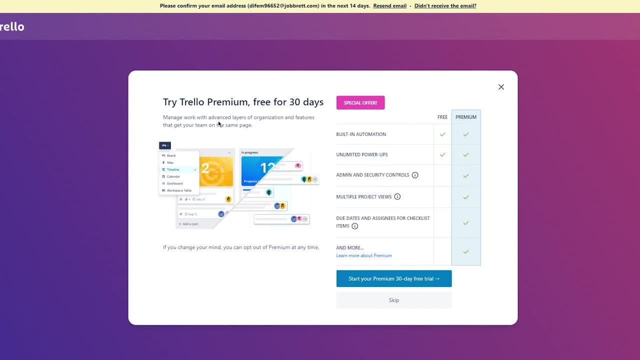 this blank for now, because we can just add this later. okay, now try trello premium for 30 days if you want to, and, as i said, you can try the whole trial, built in automations, unlimited power-ups and you know all that stuff. but i'm gonna skip this for now now, once you skip this, basically it. 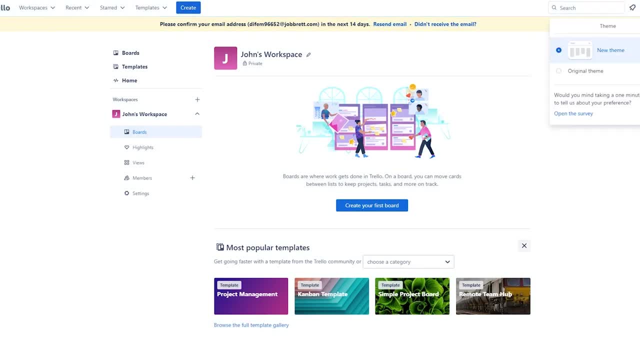 brings you to your home dashboard. now, in your home dashboard, obviously you can see all this stuff going on over here. you can see all the stuff going on over here. you can see all the stuff going on where you know. you see, john's workspace boards are where works, where it gets done in trello on a. 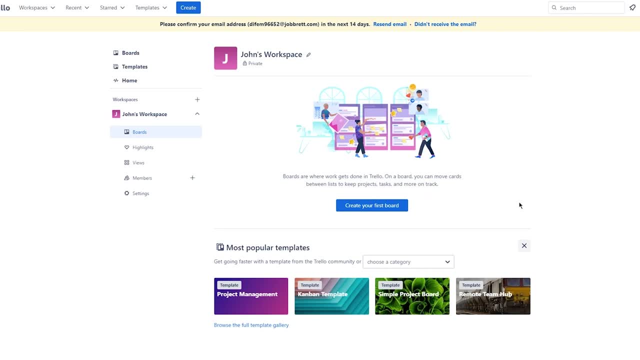 board, you can move cards between lists to keep projects and you know all that stuff. so if you were to, you know, get a brief overview of the home dashboard, here on the left hand side, you have all this stuff. you know, with your settings, the members, you have different views and all that stuff. so if 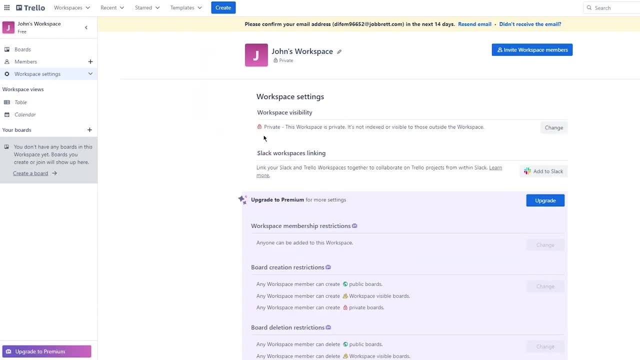 i were to go in settings. okay, here we are and over here you can, you know, mess around with settings. right now, as you can see, our workspace is private and obviously it's private because we don't have anyone in it. so to make it public, obviously you're going to have to invite workspace members and then, you know, create a link and stuff. 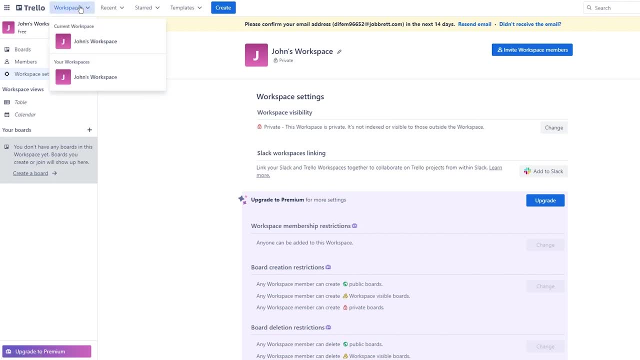 that's what's going to make it public and all things. and if we go over here in workspaces, as you can see here, you can see all the different workspaces that you have in your, you know, current email account. now, once you've, you know um discussed about you know, the workspaces that come, 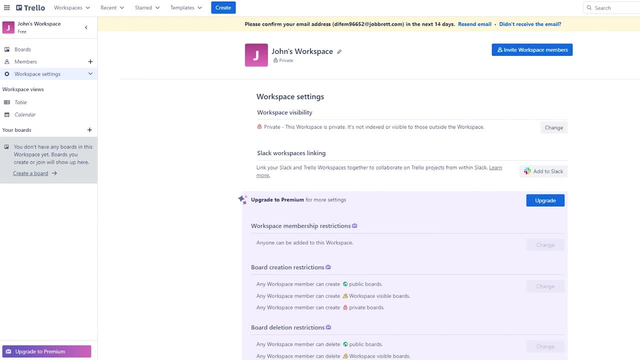 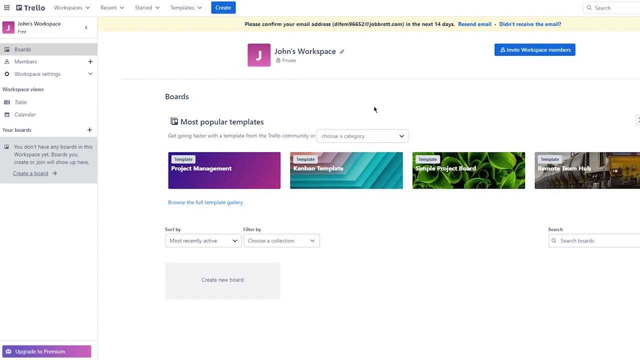 let's go ahead and discuss the boards. now. the boards are basically where you're gonna, you know, get the different um topics in and stuff. so to create a board, you're going to come to boards and click on create board. once you click on create board, as you can see it, 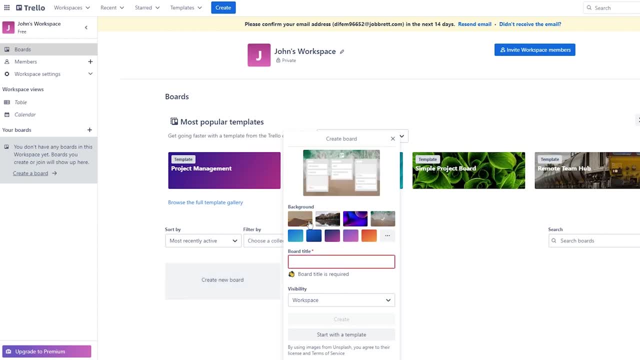 gives you a template over here. it asks you to choose a background for your board. i'm going to choose this background, uh, or you can even choose more by clicking on these three buttons and, as you can see, you get all the stuff. let's go ahead and choose that now. once you choose that, you're. 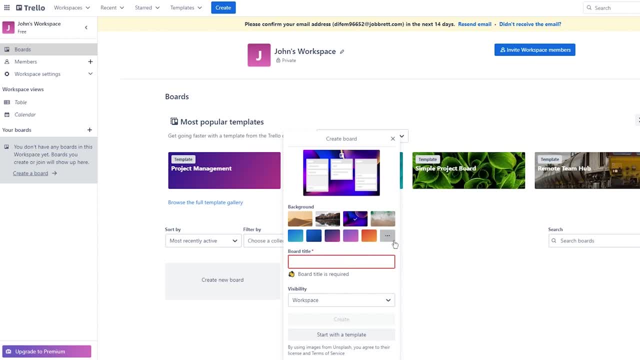 going to obviously need a board title. a board title should be you know, relevant to your company, or you could say you know the reason it was made, like you know. let's say, this board title was made for your company related to you know coding or programming, so you could say this board. 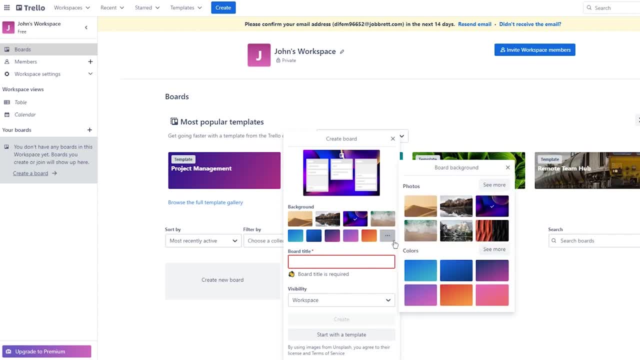 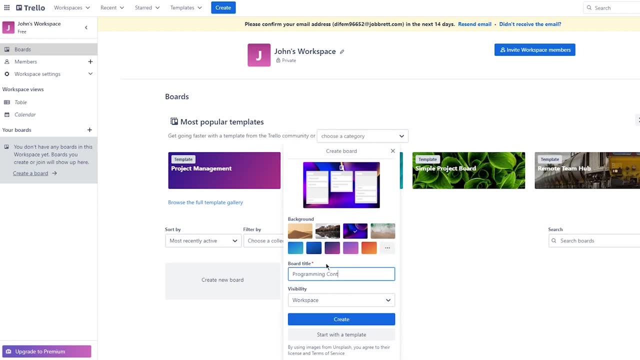 is called programming board. maybe you know something like that. uh, so here we are programming, content planning. you know something like that? call it that. then you have visibility on workspace- all members on the john's workspace. you can see this, or you can make it totally private, or you can make it public. okay, that all depends on you, obviously. 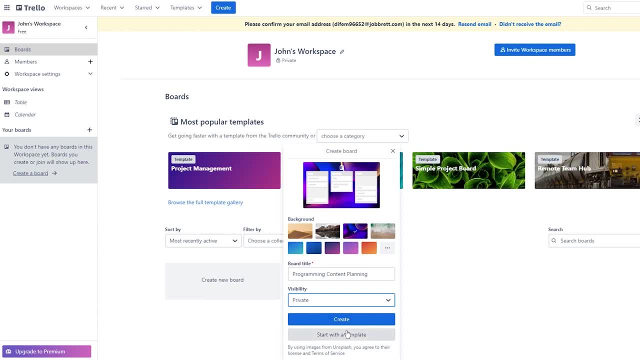 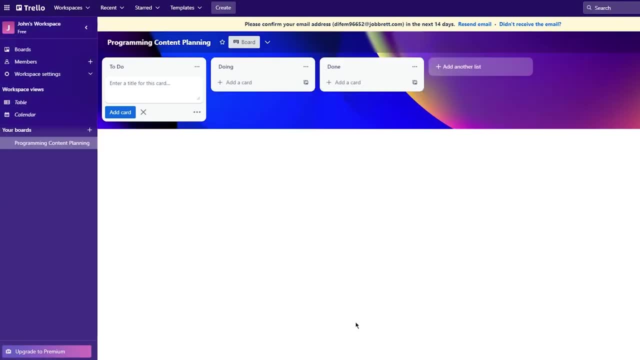 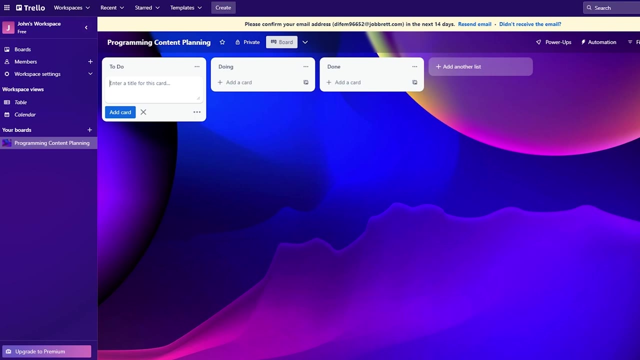 i'm going to keep it private for now. now you get two options. okay, start with a template or create. now i'm gonna just go ahead and click on create and let's see what it does. here we are now, as you can see, our board is created. so now that we've, you know, discussed boards, let's go over to 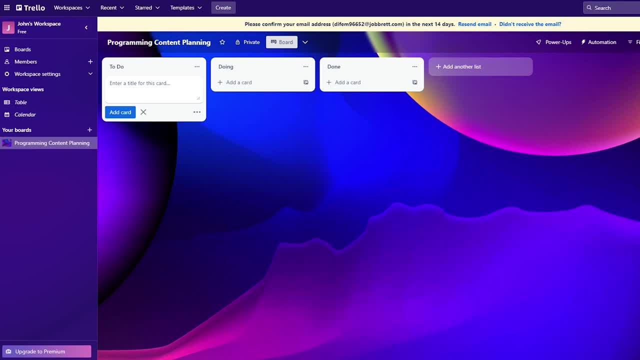 lists. okay, let's go ahead and discuss lists now. this is you know your board, where you have you know your to do, doing and done. now these are basically your lists and your boards, and you can move these lists around pretty easily, as you can see. so this is like the ease of use and you can like change this. so let's say from to do's you. 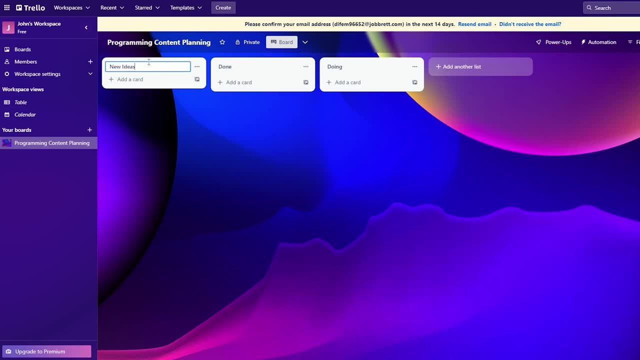 want to change it to new ideas, you know, call it that and done you can. you know implementations you can. you know, make a list over here like development, and then you can just add another list if you want to like testing. you know stuff like that. now let's talk about the content that. 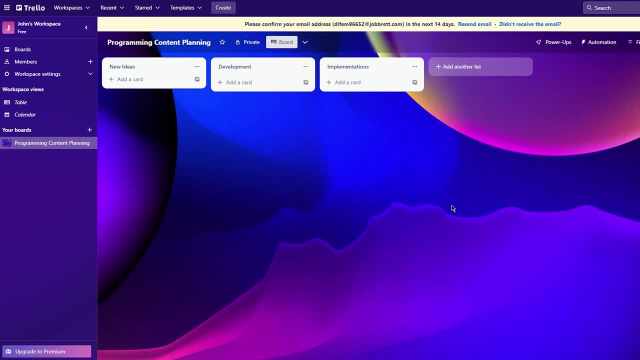 you want to add in your lists. now that i have a list called new ideas, time to add content in it. so i'm going to click on add card and i'm going to add a card. so let's say, in new ideas i'm going to write um. 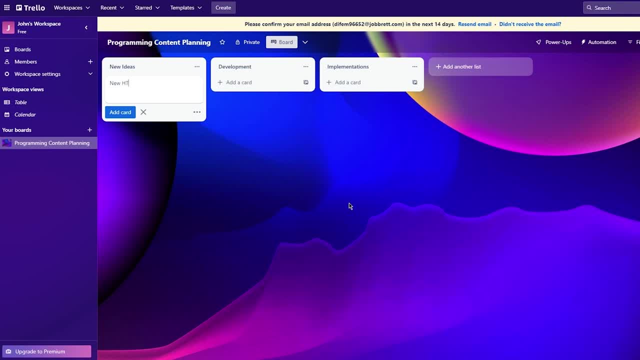 let's say, new html based app for 2023. okay, there's a card. i just added a card into my lists and, as you can see, i can move it around pretty easily, so it's pretty simple to do this. now that we've done that, let's go ahead and discuss the workspace settings. so here we are in the workspace. 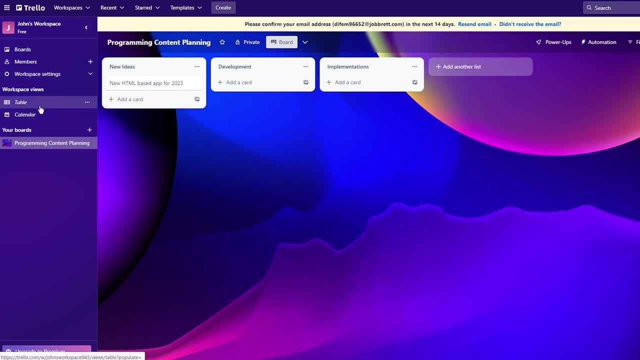 settings. you know you get all this stuff and even in the workspace views you get two views: the table here and the calendar view. now this is some gonna all work throughout the time, not everything. when you add a list, the clock is adjusted by all. you can add more keywords depending on which. 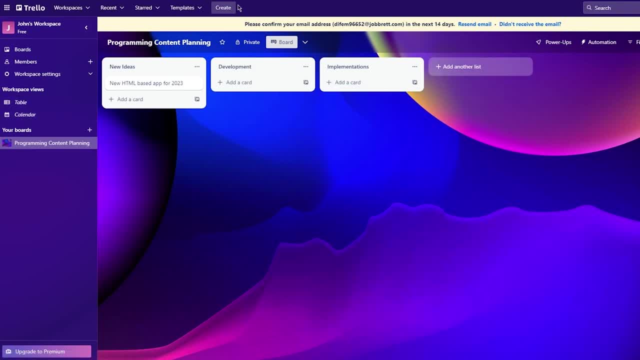 um, like the kanban view that you're in right now. so if we go on board over here and customize views, you can see you get all these different views, but to access them you're going to upgrade workspace to premium obviously. without that you cannot choose those views. now you know it's pretty. 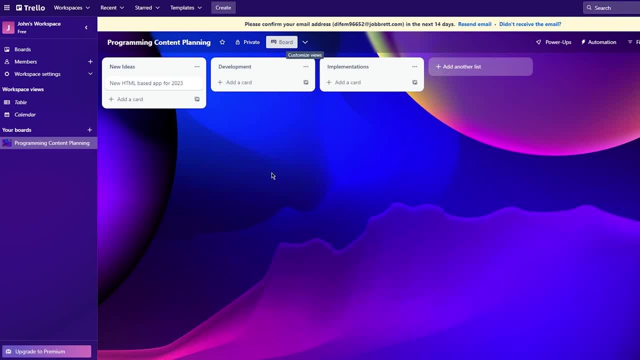 as you can see, not very difficult to you know, mess around with this stuff and if you, let's say, you want to star a board, you know, just for your ease of access, you can just come over here and click on star and once you do that, as you can see, this board is now starred. now, if you want to you. 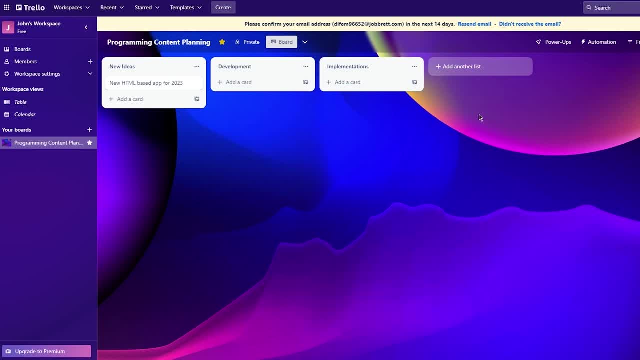 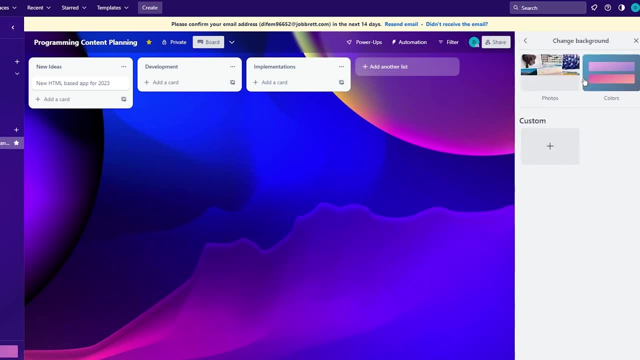 know, go more into the depth of the different colors and backgrounds that you can keep for your you know board. you can come here and click on change background and, as you can see, you get all these settings that you can mess from with backgrounds, photos, colors, and then you 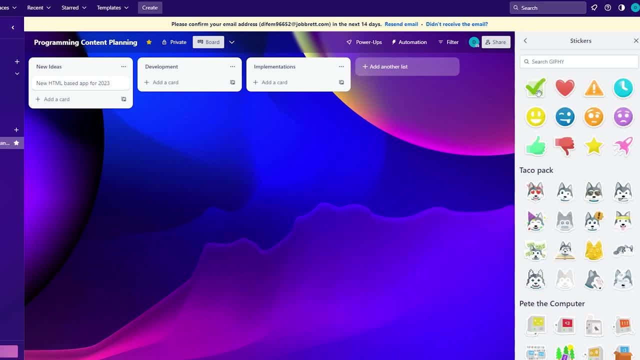 also have your default colors and you can make the settings you want to style a little bit more. also have custom fields that you can add along with stickers, like, let's say, uh, you can add this over here, you know, as a gif and stuff. and if i were to go on more, you know you get all the 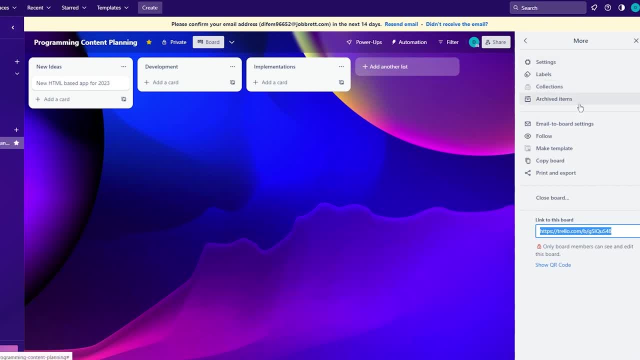 in-depth settings, like you know: labels, collections and all that stuff. this is the archived item section. this is where you're going to see, you know, your archive stuff. so if i were to go on implementations and i'm going to click on archive this list, see what happens if i go in archived. 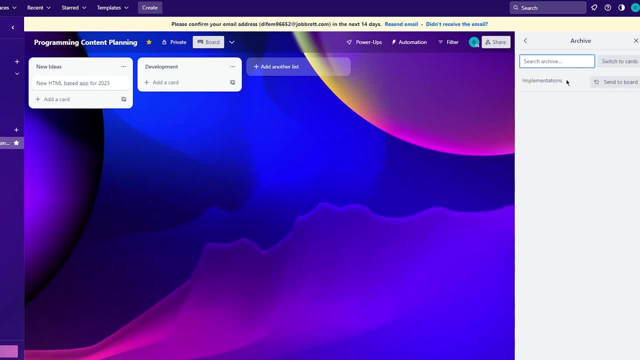 items switch to lists. look at that. the implementations is right here and i'm just going to click on send to board and look at that. that's how easy it is. then, in the same place as you can see, you have a link over here now. this link is obviously the links here- trello board, and you can. 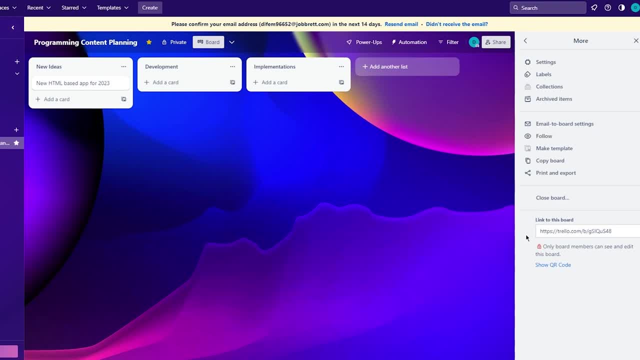 obviously circulate it around accordingly, if you want to. you know, you could say: uh, tell other people about your board. or you know, just spread your board around, tell uh, send it to your members, send it to your work colleagues and all that stuff. now that we've, you know, talked about that, 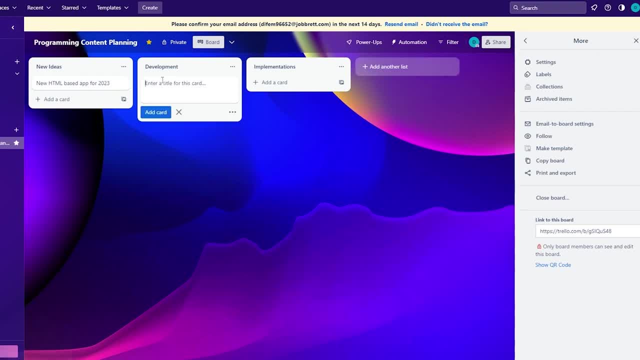 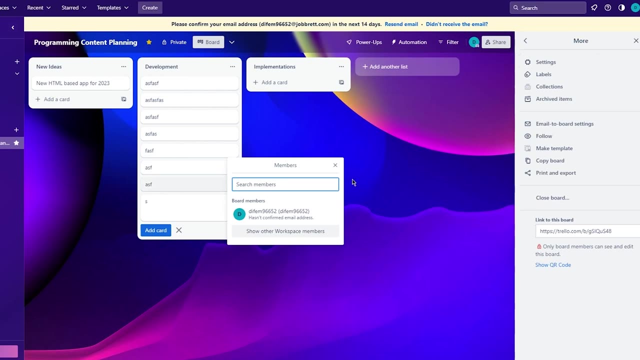 there's another basic of trello and it's how quick you can add. you know your tasks and stuff. so like, let's say you want to add a task in a speedrun, so rod something, add a task, just click on enter and, as you can see, tasks will be added pretty quickly. so let's say you have added a task. 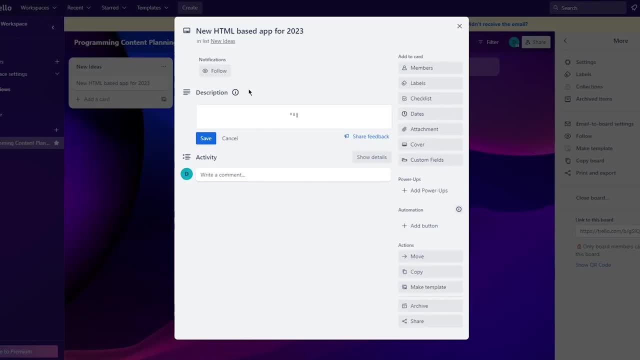 okay, let's say you've added a task, let's go, you're going to click on it. now you can basically choose the in-depth settings in this task. so first of all, there's members. these are, like, obviously, the members. you're going to choose this, what you see right now. 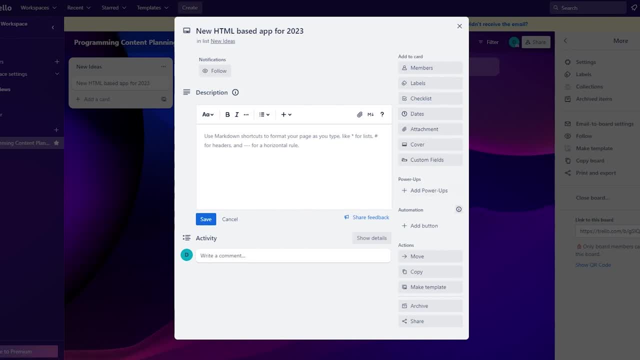 is a mastering card. this is the in-depth details that you're going to mess around with, for you know the card that you're accessing. so this is uh, you know over here, as you can see, you can change the title name if you want to. this is the add uh members. okay, add any member if you want to. 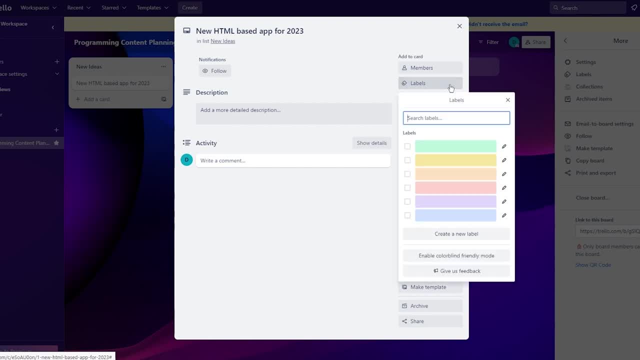 your. it's like totally up on you. then you have labels. obviously you can choose different labels for a different, you know. you could say, for different cards you can choose different labels. let's say, uh, this label means important, you know, so you can call it important. click on save. 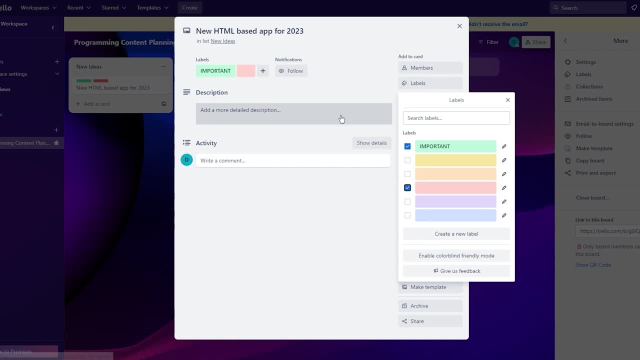 so, as you can see, this label means important, or you can also, you know, choose the red one and call it urgent and you get the point. so that's what labels are good for, and you can use them to, you know, let your people know that this is, you know, pretty necessary and you need to. 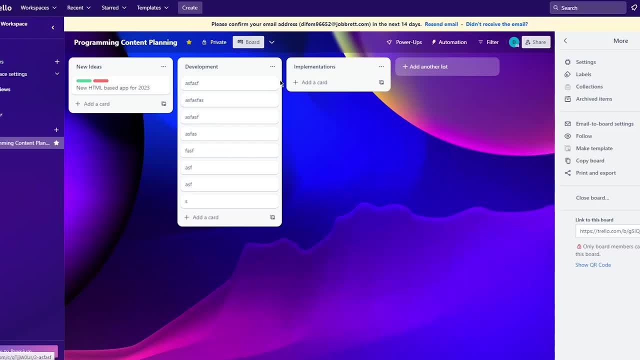 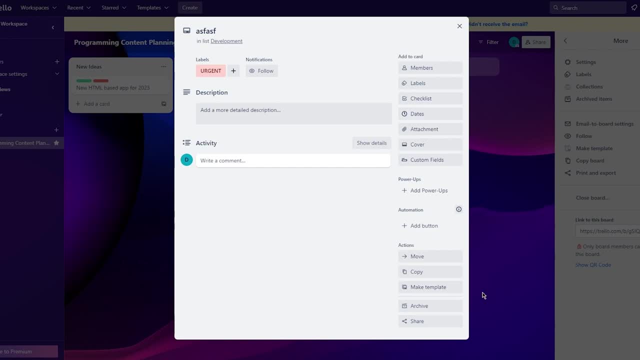 basically do this stuff pretty quickly and then from there on out you can basically add it pretty easily, like click a task, click, go on labels and look at that, just add it over there. so that's how simple it is. it's pretty easy. uh, then obviously you can. 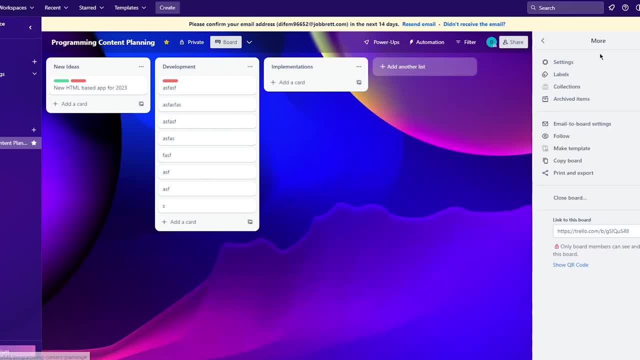 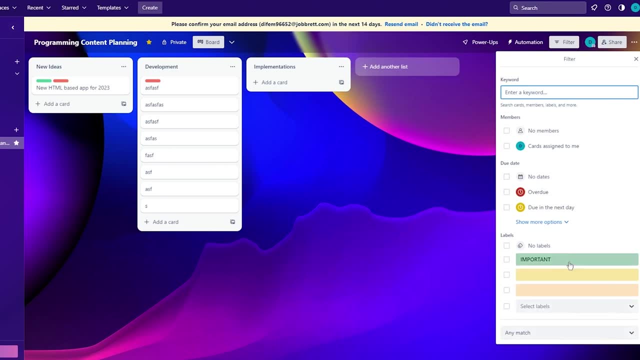 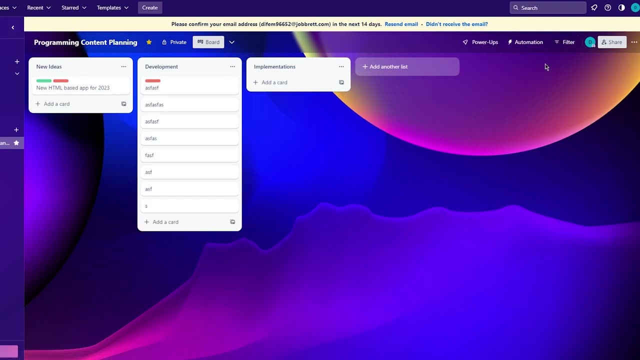 also like filter things out accordingly. like, let's say, you were to go over here and you want to filter all the urgent ones out, so you're going to go and filter and you can obviously select a label, go on urgent and look at that, it filters all the urgent ones out. so that's a pretty cool thing to 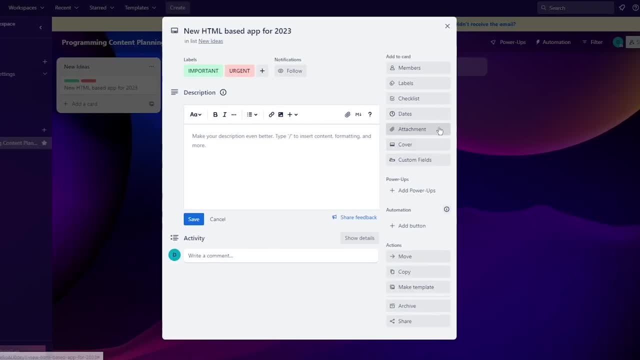 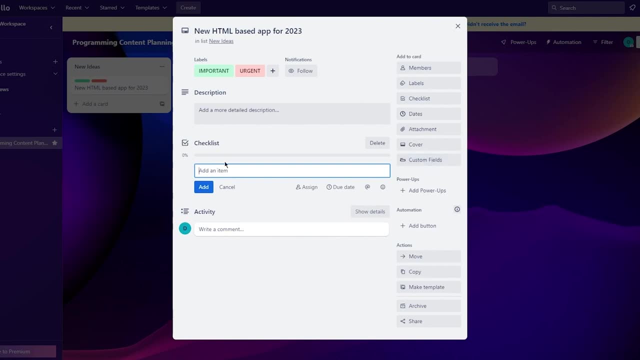 have as well. then you can also add checklists. so if you were to go here- title checklist, i'm going to add that. look at that. you have a proper checklist now and you can start adding items. so you can start, you know, maybe telling people what they're going to do. so you have the 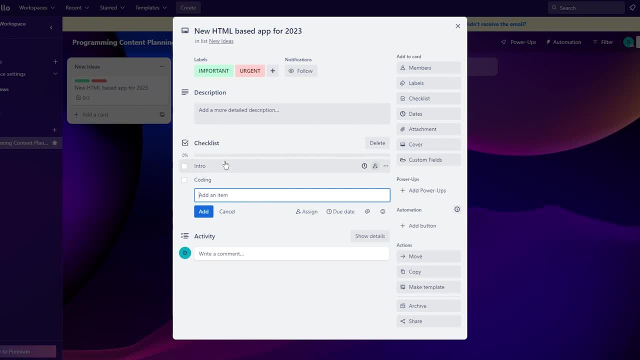 intro. you have the coding, you have understanding, implementation, development and then testing. okay, let's call it that. so these are basically your checklists and a person like when they're doing this task, they can, one by one, come here and, you know, check these in that. yes, i'm done with this. 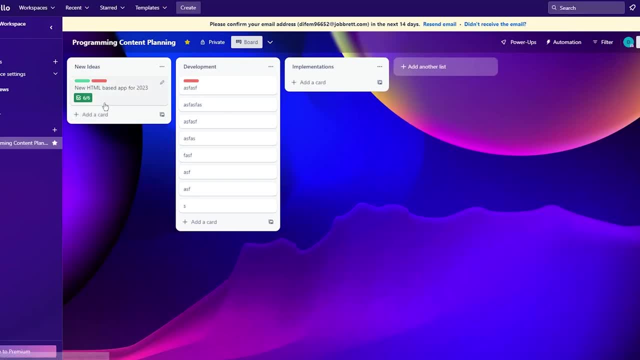 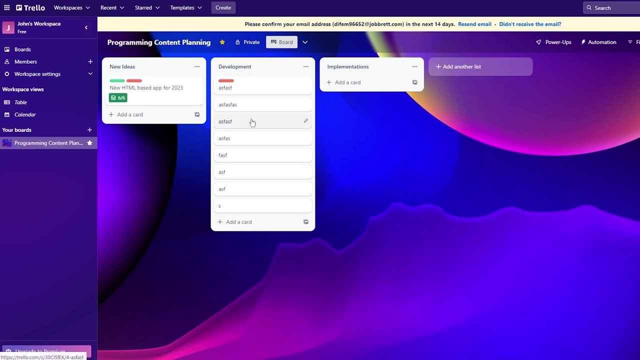 i'm done with this and you know all that stuff. so once all of these are done, you can obviously come here and see that, okay, this person is done with these things. that's good. so that's like again one of the ways. so let's say, you have a task over here and you 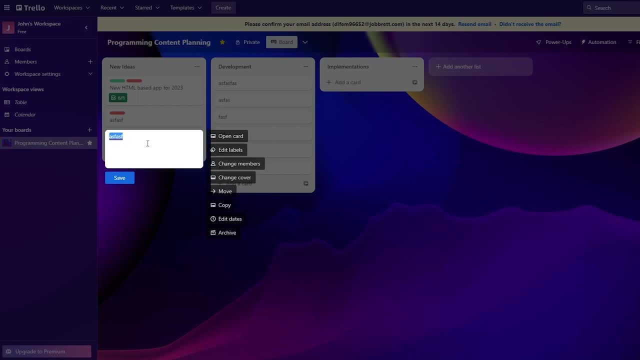 want to mess around with it. you can right click on a card and once you go over there, as you can see, you get like a quick menu opened over here. you can edit the labels, change members, you can also change the cover of this card. you can also archive it directly from here if you want to, as 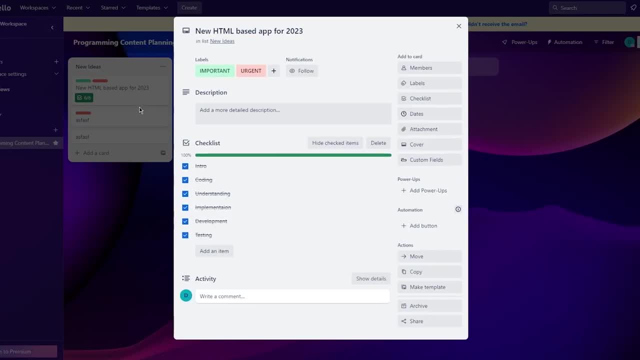 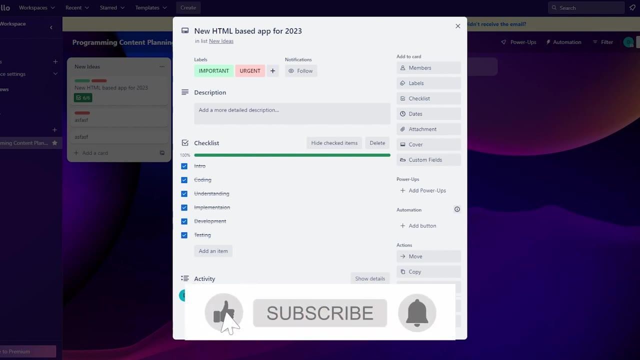 i told you earlier on. now, let's say, you have the checked one over here. uh, you can hide the item. show the check items for yourself, if you want to. you can also add a new checklist, if you want to. again, totally depends on you. then you come over to dates. okay, now in the date section. wait, let's. 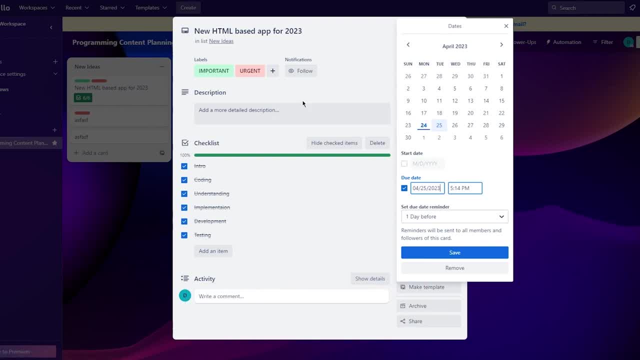 head over here in the date section. basically is when you set the time limit for a certain, you could say um task on the card. so let's say this task for the new html based app for 2023. let's say a time limit for you. we don't want, we like, as i said, it's pretty important, it's pretty urgent. 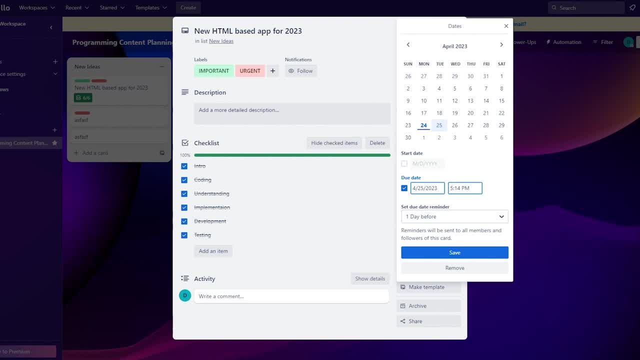 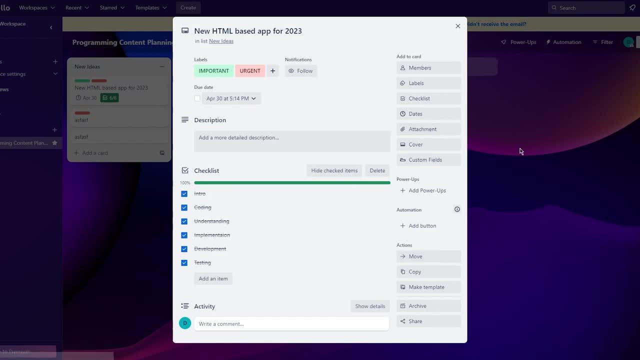 and we want it pretty quickly, so let's set a time range for it. so let's set it from 24th to the 30th. that's the time range. i'm going to click on save and once you click on save, as you can see, april 30th is the last date and um 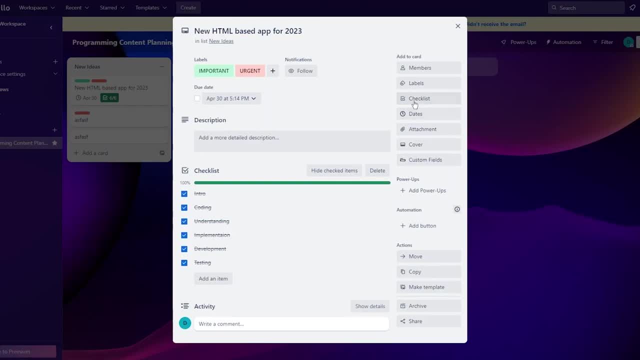 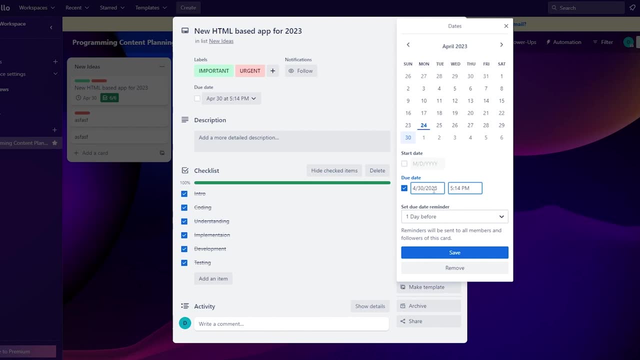 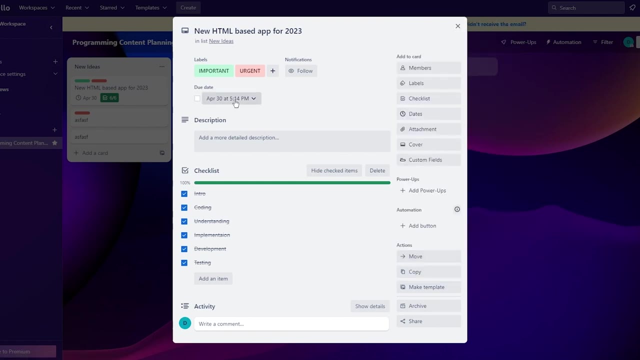 it shows it over here and that's like a pretty good thing about it. and also you can like set the due. the due date has been set, but you can also set like the exact time you want it and um once you like do that, you can click on save and, as you can see, you have a proper due date and 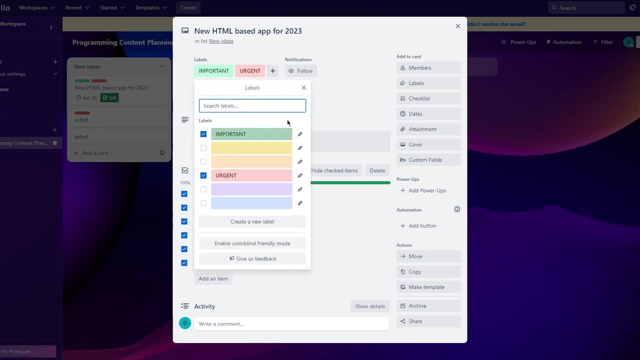 time. now you can also show more labels by just clicking on this plus icon if you want to. as you can see, more labels can be shown accordingly. now one more thing like, let's say, you want to give reference of a media to a task, so to do that, what you can do is you're 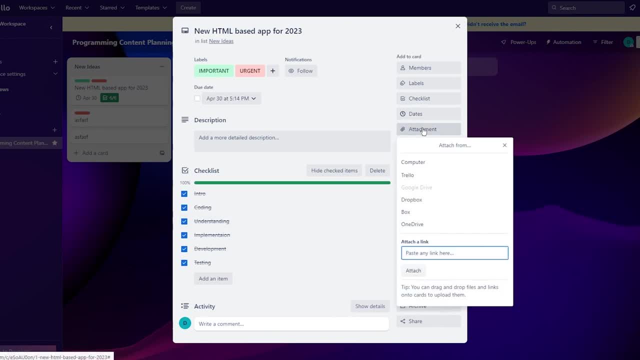 going to go to your media and you're going to click on attachment and you're going to click on attachment. if you go in attachment, as you can see, you can also paste any form of media into your trello board to give your user a um reference. so let's say, if i were to go on computer, look at. 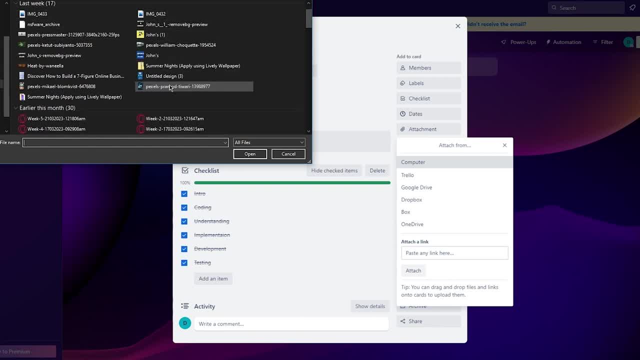 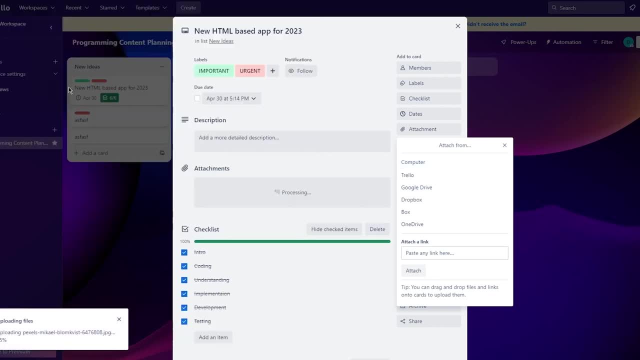 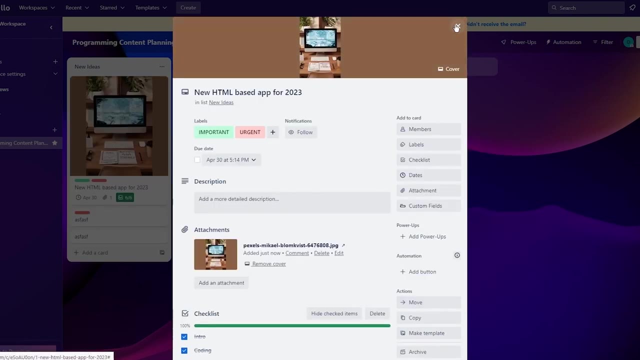 that you can choose all these images from your computer and paste it onto your- you know- trello board. so let's go ahead with this. let's just add this photo randomly. as you can see, it starts up a little bit and then it starts uploading your file, and once the file is uploaded- look at that- it adds: 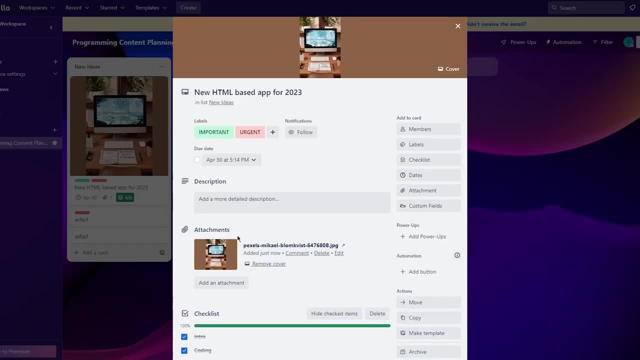 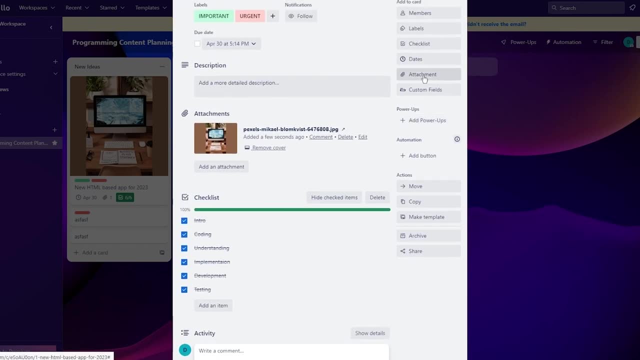 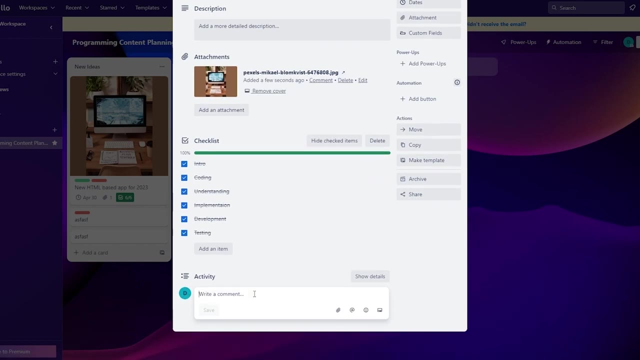 that as a cover photo and look at that. it's right there. and if a person clicks on it, look at that in the attachments. they can see that as a cover photo and you can also like paste it in the comments down here if you want to. so let's say, if i were to copy its link address, you can just come down. 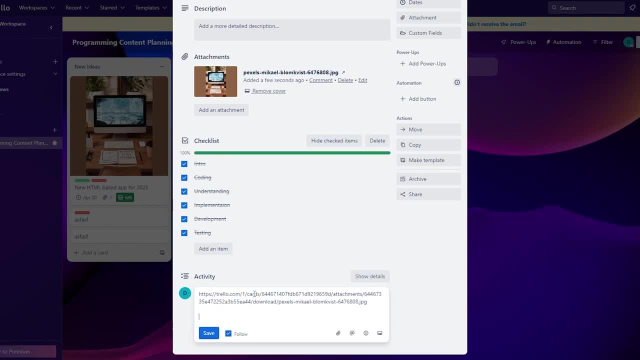 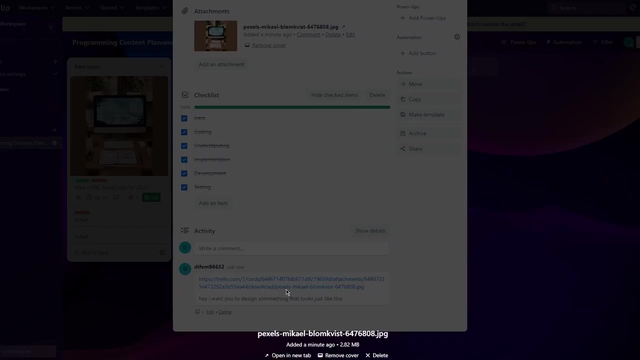 here and be like, you know, paste it and, you know, add a few space and be like, hey, want you to design something that looks just like this. okay, you're just gonna write that and click on save. now, once you click on save, look at that: um, people are, you know, gonna click on it. 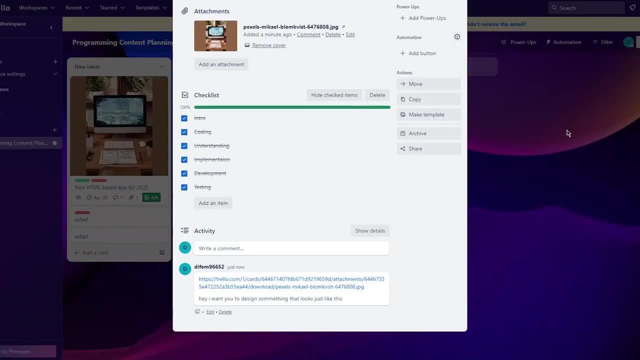 and look at that this image is gonna open for them. so it's pretty easy to work around with this and people you know can add emojis to let you know that. okay, we, we've seen your message and uh, you know it's all good, they can send you a thumbs up and uh, you can. 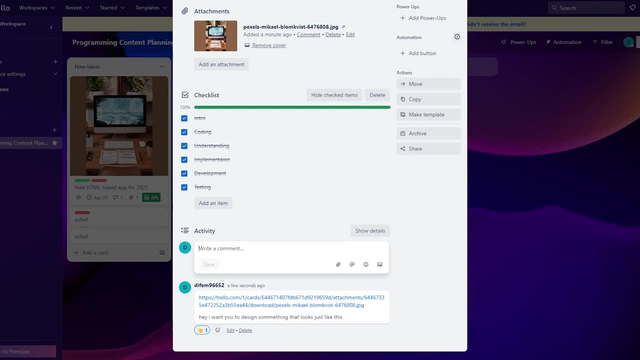 also like tag a person, if you like want to, you know, specifically tell someone and notify someone that you want their attention, you can click on at you know, put in their name and once you do that, just write something and that's going to add them and basically it's gonna call them in that hey. 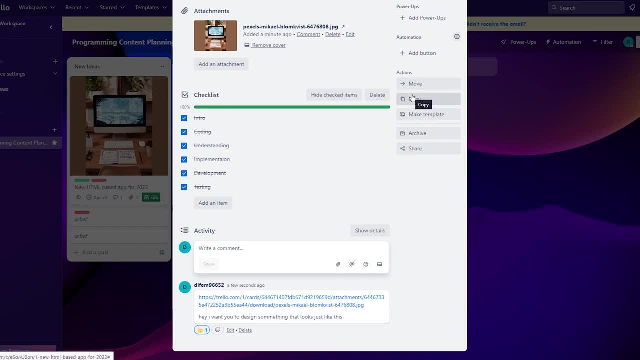 i'm letting you know that this job is pretty important for you, so please check this trello board as quickly as you can. also comes the move card, where you can like move this into. you know different cards if you want to. so, as you can see, i moved it to development. 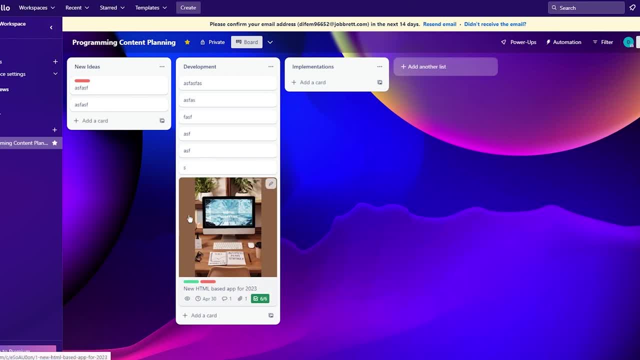 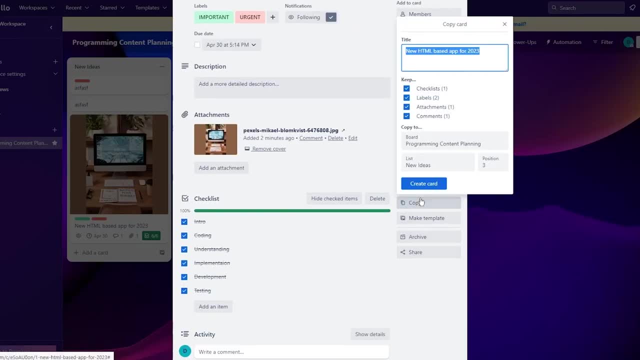 and it's right here. but you can like not do that. you can just do this for the moving. it's pretty simple and obviously if you open again, you can also copy a card. okay, and you know, implement it and paste it in some other place if you want to. uh the copy- basically you know copies the whole. 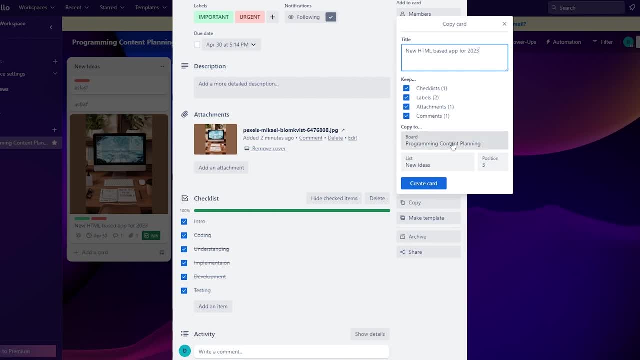 title with the all the checklists, labels, attachments, comments, and then you can copy it to a different board and you can also choose the list you want to copy it to. so let's say i'm going to go and create card. look at that, it creates a copy of another card with 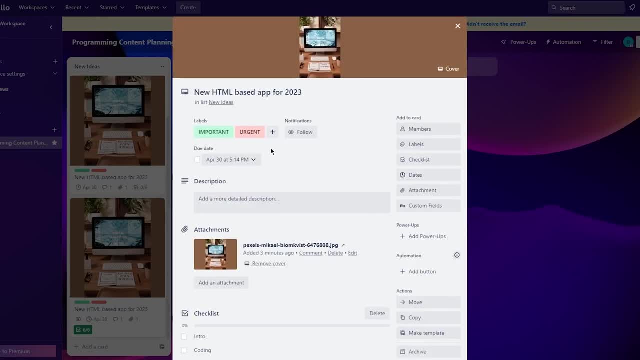 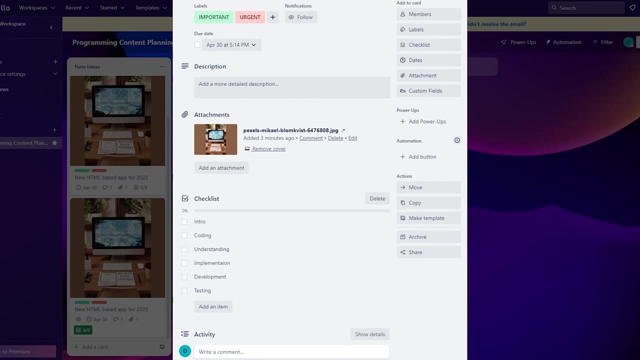 all the same things, including, you know, the checklist and everything, and that's the cool thing about this- like it's pretty cool, it works wonders. so, yeah, it's pretty fun to do that and it's a good thing to you know, have by your side and work around with now. 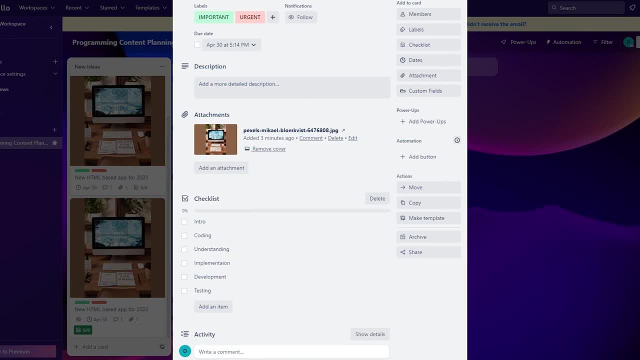 you can do more with. you know the privileges you have on trello and we're going to be discussing all of that as well. so, again, we've discussed about cards, we've discussed about lists and how you're going to, you know, fill them in and all that stuff. so let's go ahead and 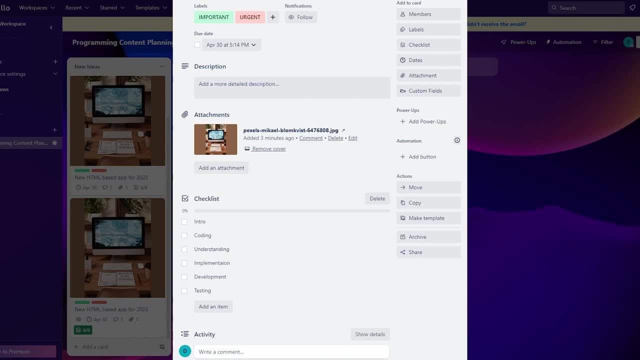 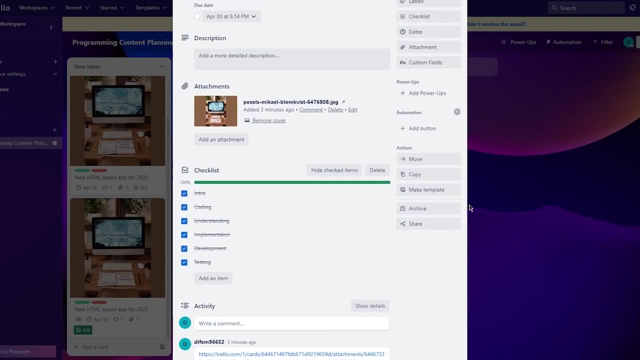 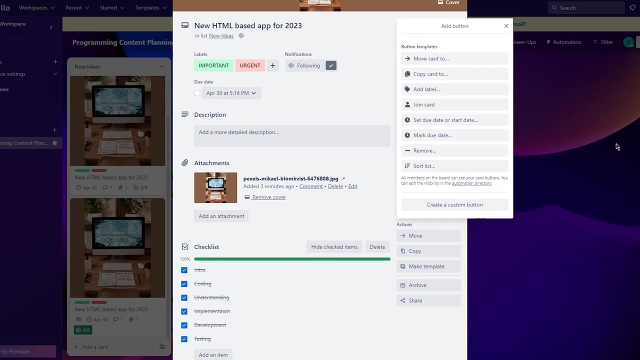 you know, discuss about the watch feature when it comes to actions. now, the watch feature basically comes when your you know, uh, let's say, trello card is fulfilled and done, and it basically comes by adding yourself some buttons or power-ups. okay, now the power-ups could be: you know anything for? 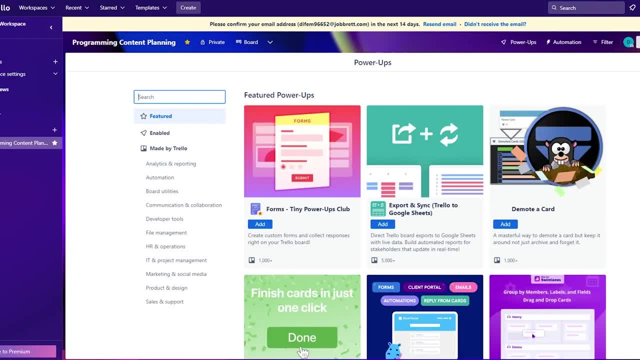 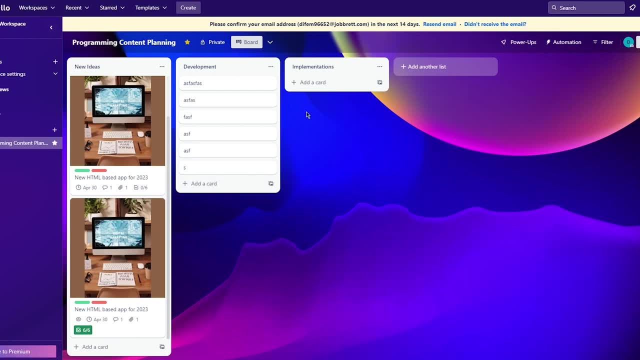 fun or anything that uh could be useful as well, and we're going to be discussing power-ups in like a few seconds, so uh, basically, trello power-ups can be pretty useful to you. okay, trello power-ups, have a, you could say a little bit more power-ups. 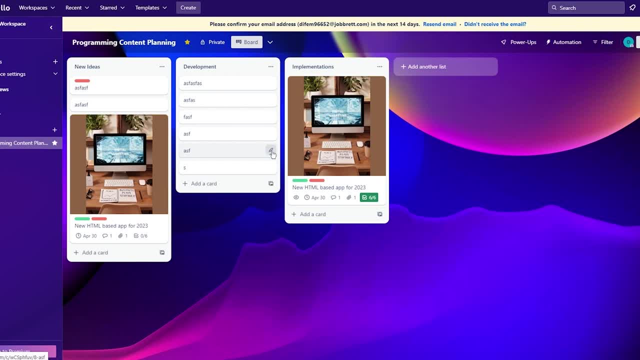 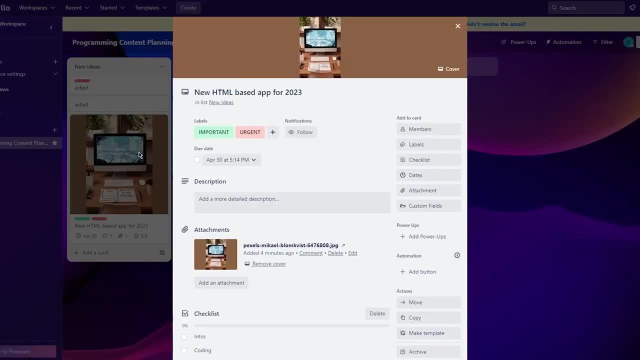 a great deal of importance because they help you easily do things. they help you access things much easier when it comes to trello. so let's say, if i were to go on this task over here and click on power-ups, you're going to be, you know, redirected to power-ups or you can just 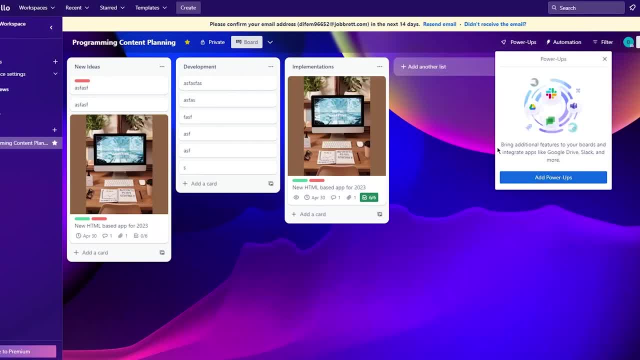 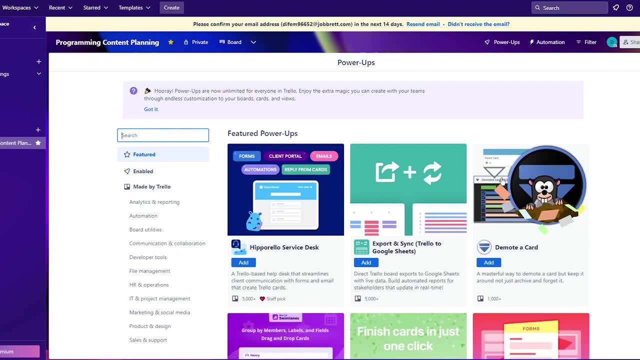 come here in the power-up section and look at this, bring additional features to your boards and integrate apps like google drive, slack and more, so we're going to click on add power-ups. okay, now, once you click on add power-ups, you're going to come over here and, as you can see, you're. 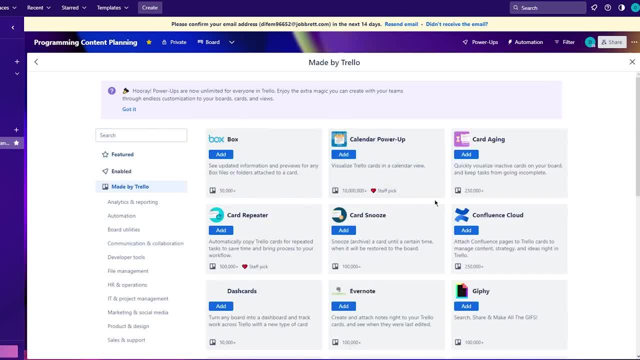 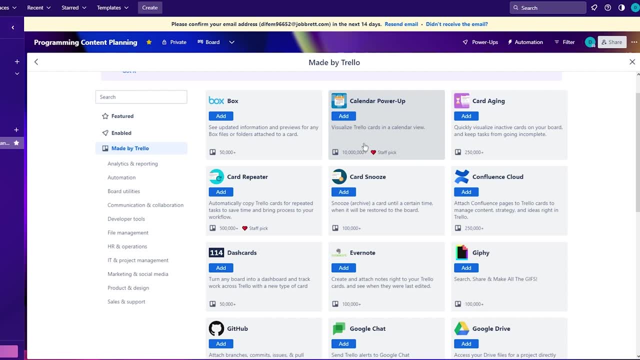 going to get all these power-ups if you go on- made by trello, you can get all these different power-ups that trello made themselves. so look at that calendar power-up. visualize trello cards in a calendar view. then you have github: attach branches, commits, issues and pull requests to. 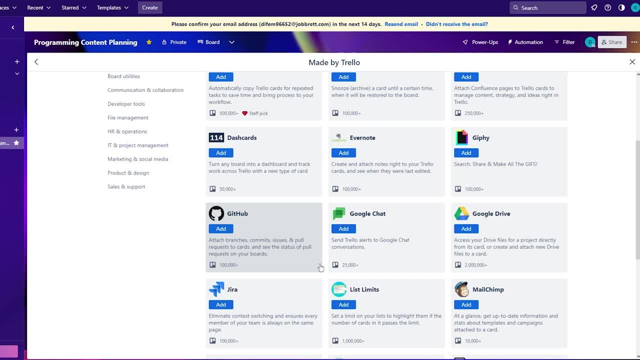 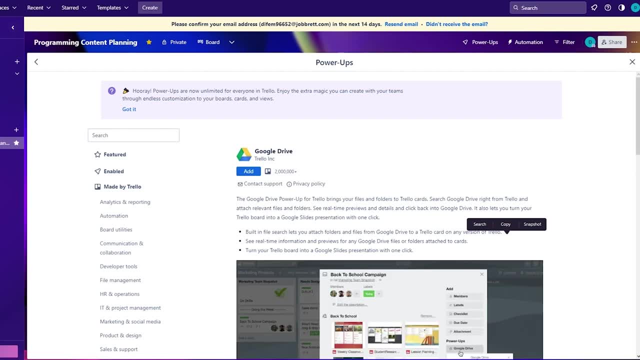 cards and see the status of pull requests on your boards. then you have google chat. send trello alerts to google chat conversations, access your drive files for a project directly. you know all that stuff that goes on. now, all these things that we're going to be talking about today are going to be: 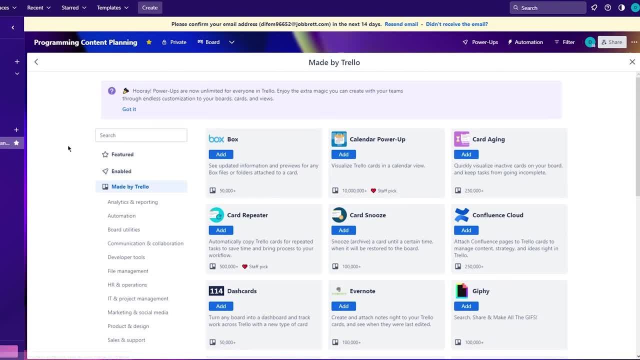 going to be talking about today are going to be talking about today. are going to be talking about things that you see, basically power-ups can also be called integrations. okay now, if you don't know what integrations are, integrations are basically when your you could say, uh, one app connects to. 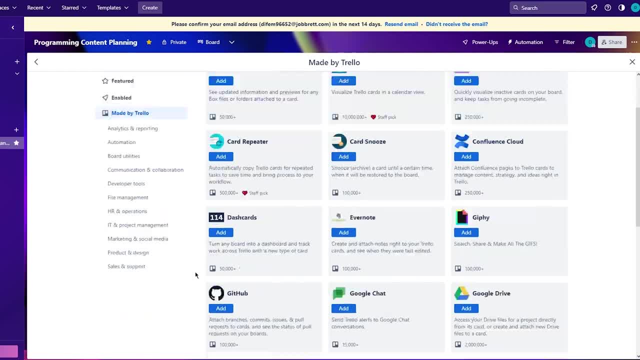 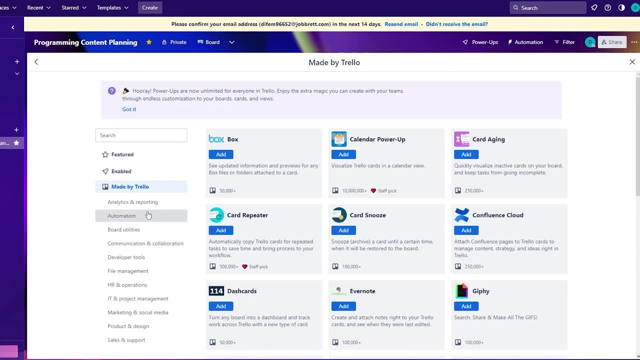 another app to make it, you know, easier to work around with. so that's what integrations do and, uh like, in my opinion, using them wisely, uh, along with your project management board, it could be, you know, pretty useful. so just go ahead and, you know, explore things out for yourself, see what works best for you, because, 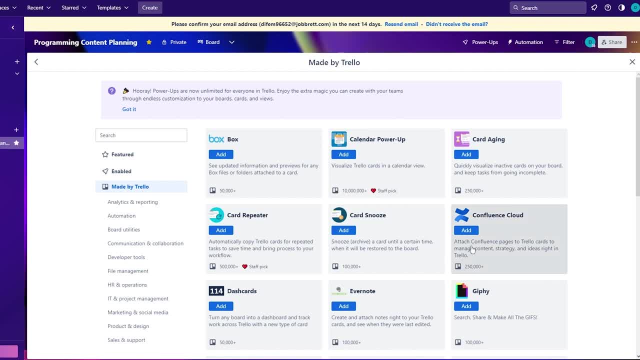 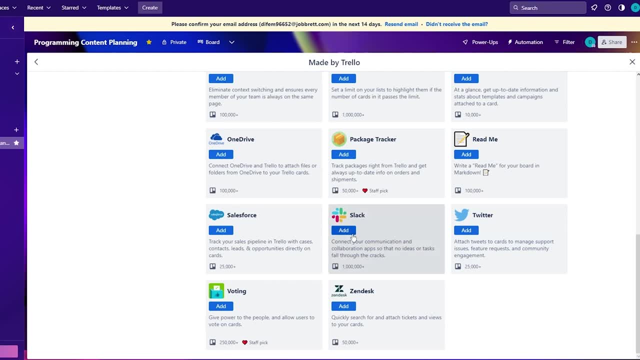 when it comes to, you know again, as i said, using these uh power-ups wisely, it makes life pretty easier for you, like pretty much easier for you, and the the most widely used ones are, like you know, voting, give power to the people and allow users to vote on cards. so, as you can see, it has over. 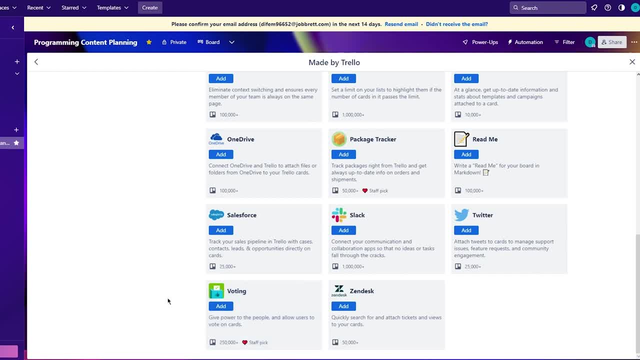 250 000 plus downloads, and people add these because they're using these cards. and they're using these cards because, um, like, let's say, if there's a task or a card and you want approval on that card, that okay. should i go ahead with this card or should i not? please give me your opinion. 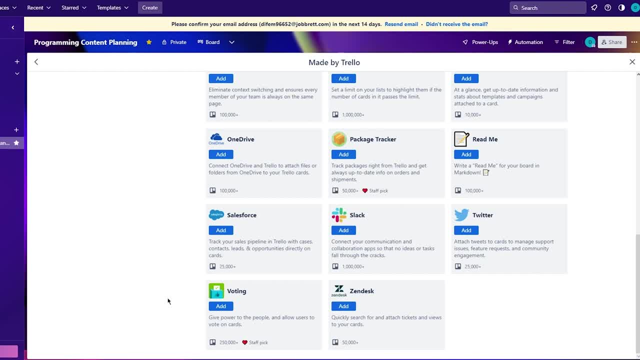 you know, you can ask an opinion like that and once you do, people are going to send you out their opinions and be like: hey boss, this we don't, we're not really sure about this, or they can, you know, have a whole debate around each other. so it's a pretty good democracy system and it's a good thing. 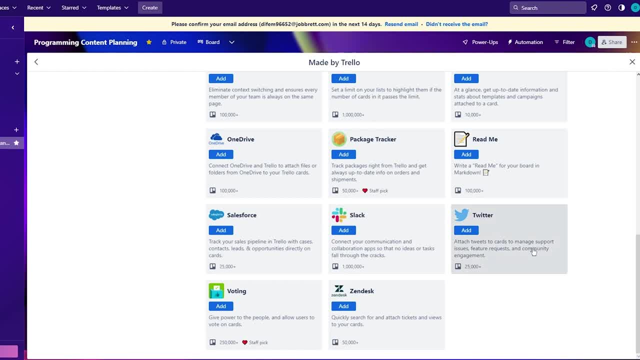 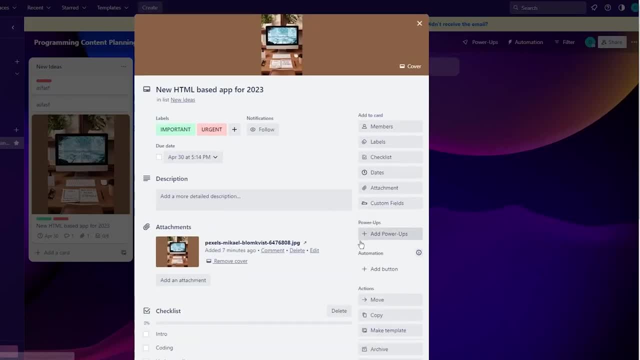 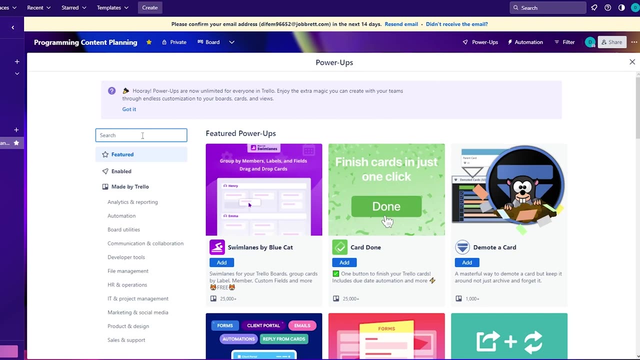 to be able to add to your- you know you could say uh- cards, because it just keeps the workplace very professional. so again, if i were to go over here, i'm going to click on add power up, okay, and once i click on add power up, we're going to come here. now. remember where you saw it go on: made by trello. 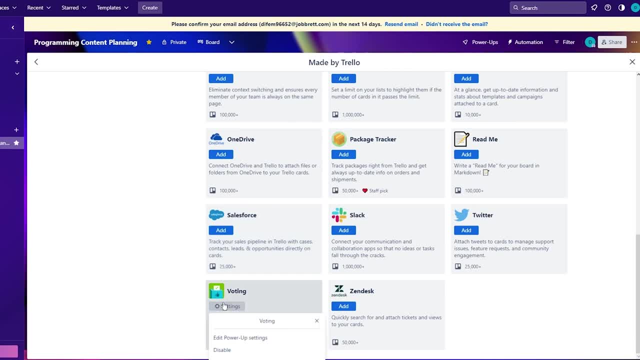 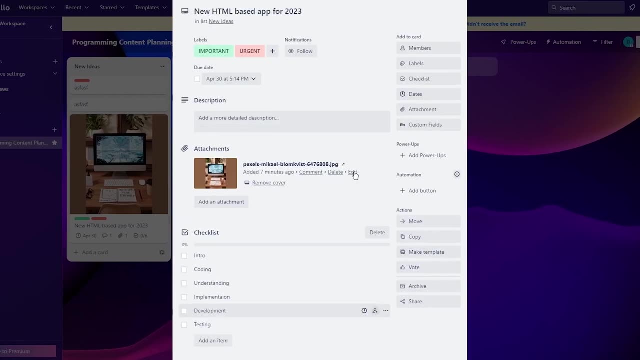 come down here. here you have voting. i'm going to click on add. go on settings. you're going to edit power up settings. who is allowed to vote on the cards? you can choose whoever is, and once that is done, yeah, you're good to go. so you just added a power up to your card. okay, now that is you know. 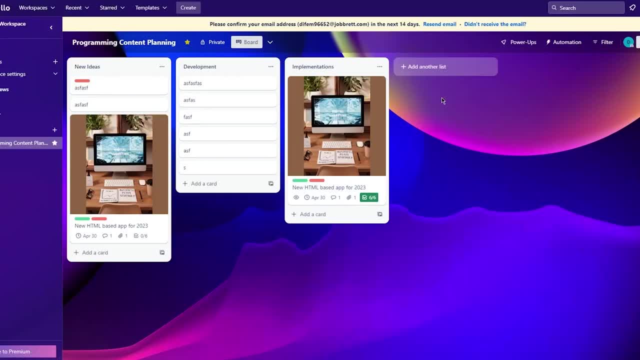 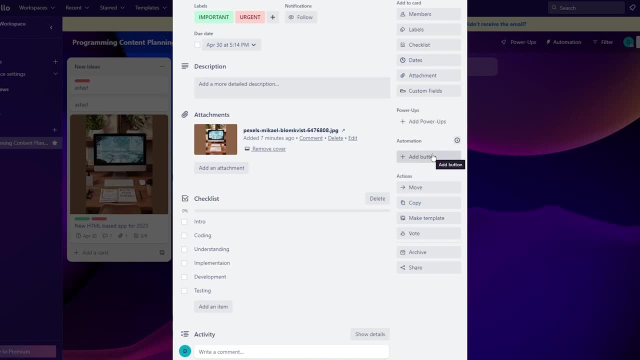 how simple and easy it was to add a power up now to basically do the voting on this power up. basically, again, you're going to make sure to set like the custom fields for yourself. so once like it's set for your team, like you've set your members, obviously, then there's 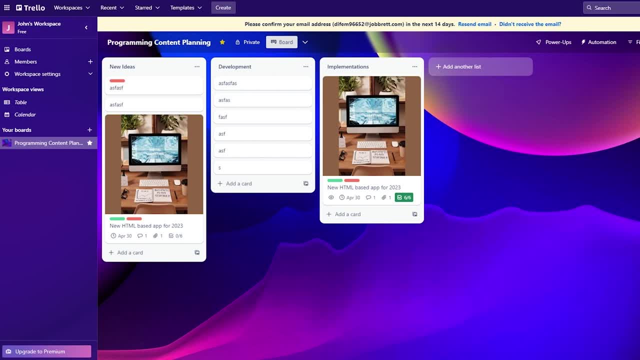 nothing you can do with it because obviously you've set it for your members. it's only for your members, so just set the power up and move out of it. now that we've discussed integrations, let's go ahead and discuss automations. okay, now, if you don't know what automations are, basically, 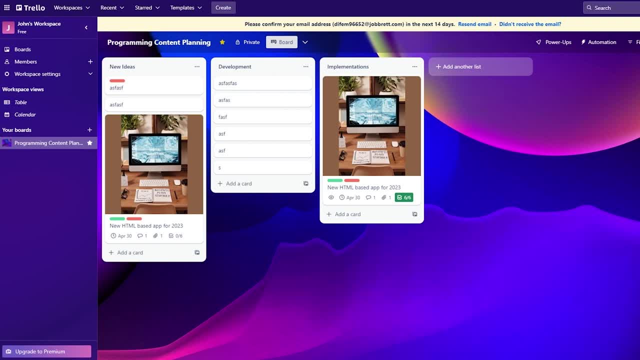 automations are when there's like a trigger in a video or a trigger that takes place, an action that takes place and that triggers another action. okay, that's what it basically means, so you could do that. so, if you want to do that, hey, you've made a purchase on an online store on an online store. 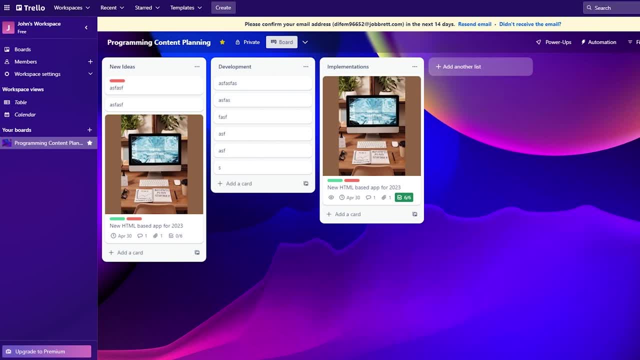 now, once i've made the purchase, what's going to happen is i'm going to get an email in like five to ten minutes that, hey, you made a purchase from our store. can you confirm this order? that's automation. so basically what happened was i did an action which was purchasing something from an 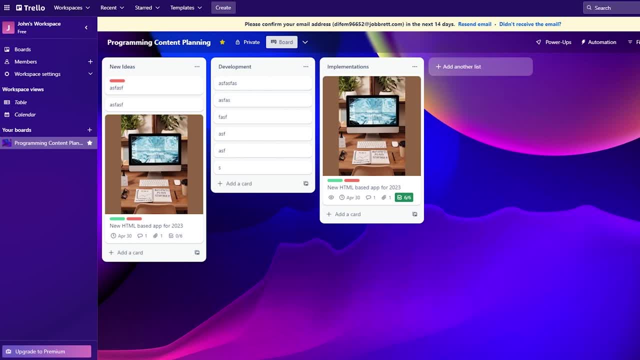 online store and the like. that was an action. for me, the trigger was that that triggered the email system to basically send me an email regarding the order. so that's basically what automation is, and that is what we're going to be setting up for our trello, because it is equally 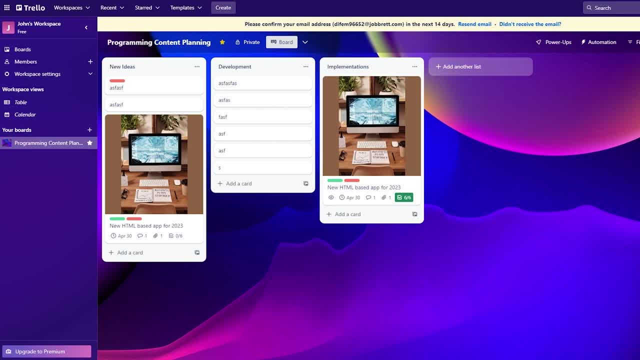 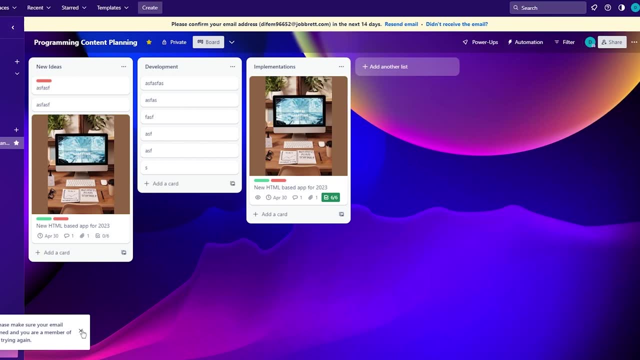 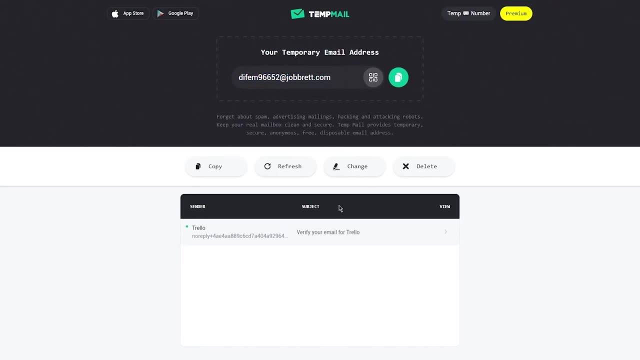 necessary, uh, when it comes to, you know, having a successful and working project management board. so we're going to go on automation over here again now. to basically work with automation, you're going to have to confirm your email address, so i'm just going to go ahead and verify my trello. okay, uh. 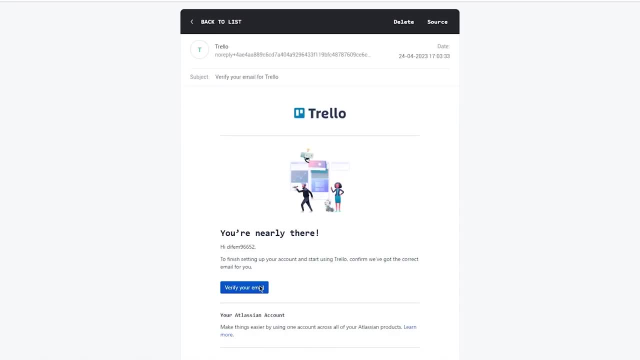 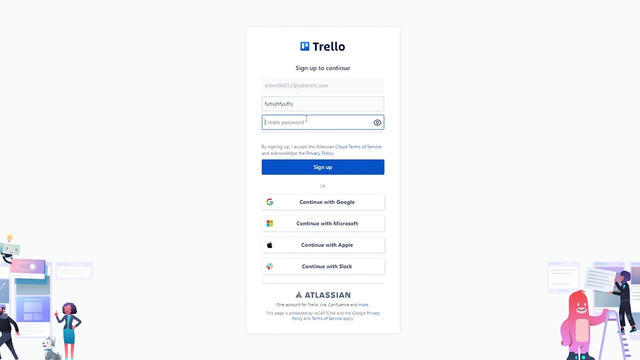 so verifying your trello is pretty easy: just check your email. it's going to say: you know, verify your email and stuff, and once you've done that, just choose your full name. okay, once you do that, create a strong password for yourself and once you're, you know, fully done with this. you're. 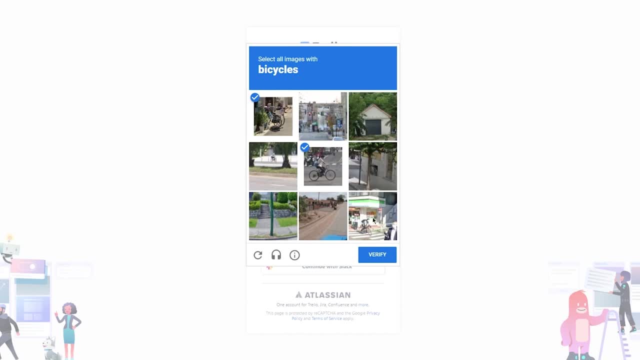 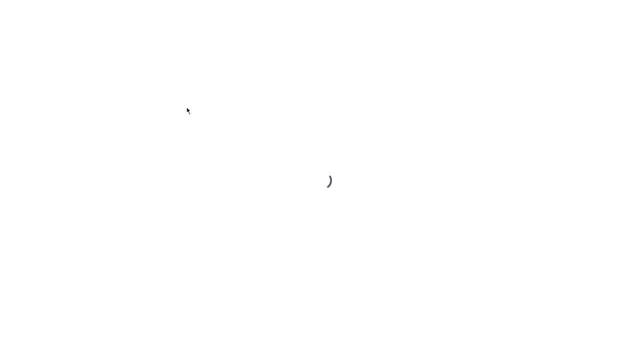 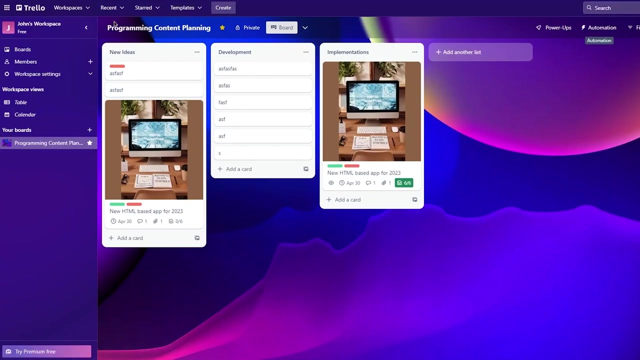 going to easily be able to use. uh, you know your automations and, just you know, make life easier for yourself. so, once you're done with this, verify yourself. and yeah, here we are. so we've authorized ourselves, we've logged in and I'm just gonna come here, I'm gonna reload the page and, as you can see, we 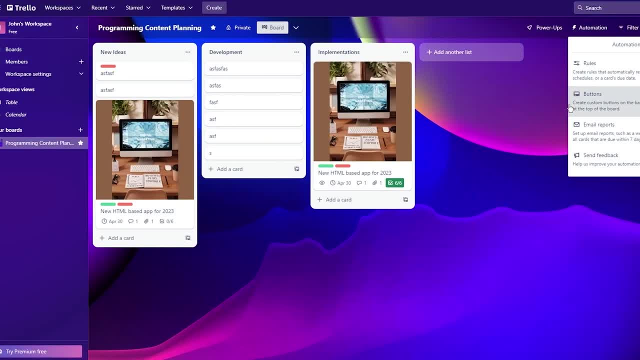 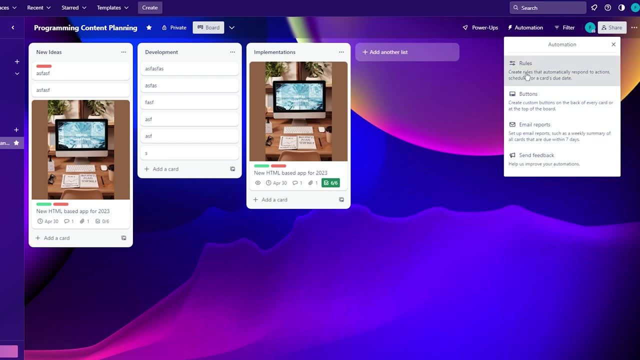 have been authorized and verified. now, as you can see, we can access automations. now, once automations are, you know, easily accessible here you can see, automations have different things around it. so, first of all, you have rules. you can create rules that automatically respond to actions, schedules or cards, due date then 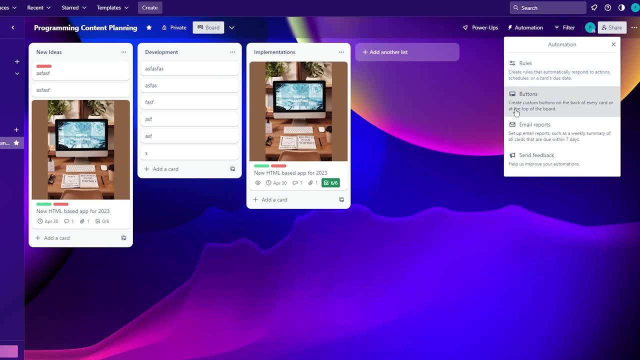 you have buttons, where you can create custom buttons on the back of every card or at the top of the board. then you have email reports, where you can set up email reports, such as a weekly summary of all the cars that are due within seven days, and then you can, you know, do a send feedback where you can help them improve. 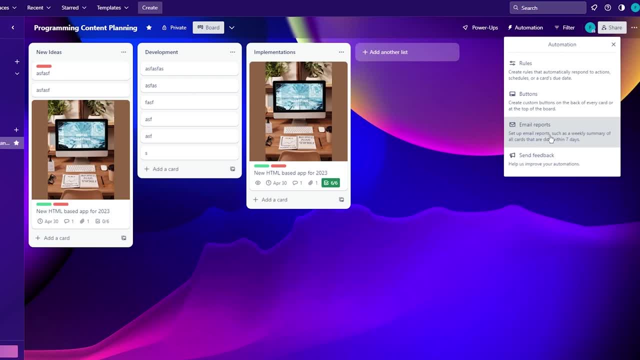 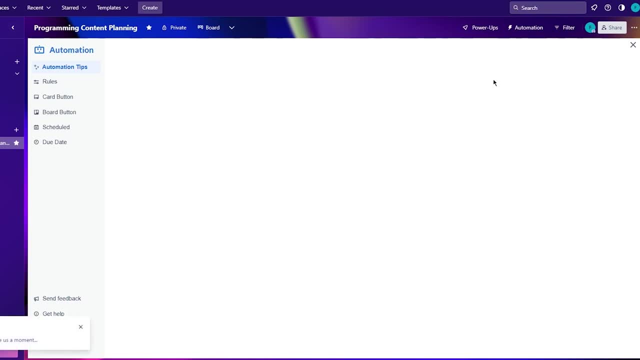 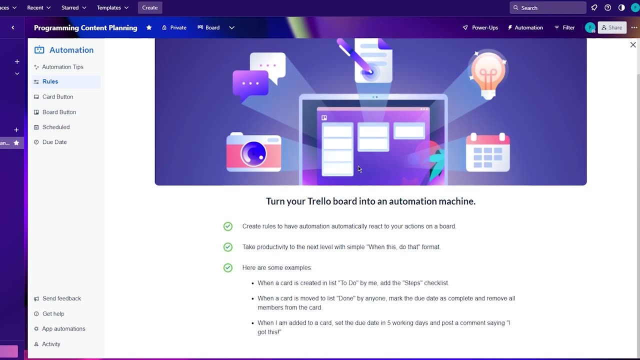 their automation. all these features obviously have their own- you could say- taste. so I'm gonna go on rules, okay, and once you go on rules, as you can see over here, they're gonna give you all of this. so turn your Trello board into on an automation machine. 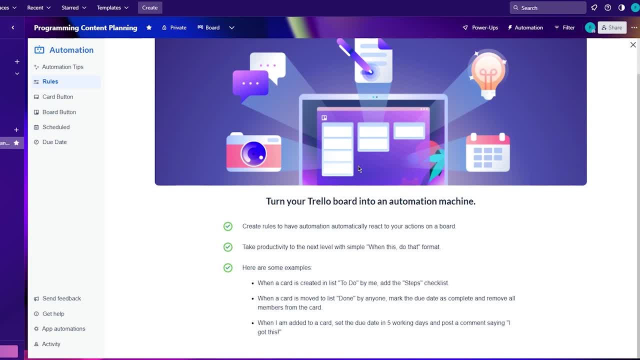 create rules to have automation automatically react to your actions on a board. take productivity to the next level with simple when this, do that format. here are some examples: when a card is created in list to do by me, add the steps- checklist. when a card is moved to list done by anyone, mark the due date. 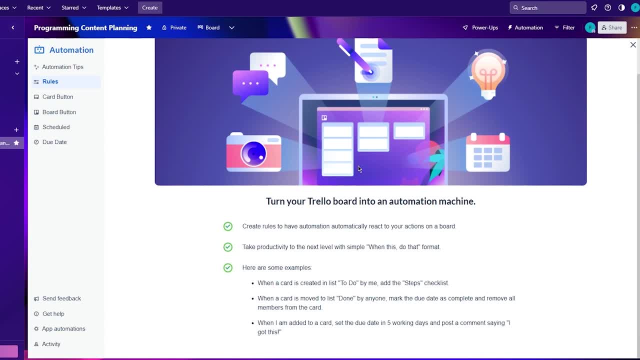 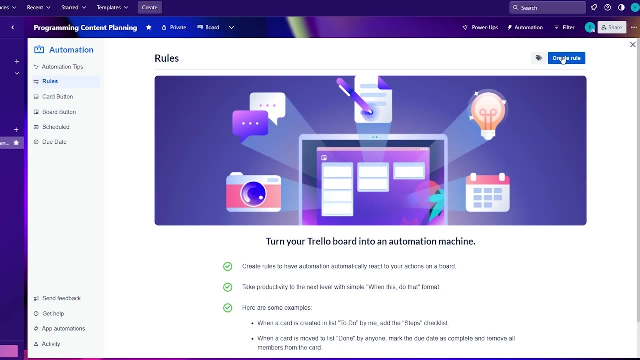 as complete and remove all members from the card when I am added to a car to set the due date and five working days and post a common saying: I got this. so you get the point. you get what you know. your automation, their basic look into you. so when some here, I'm gonna go ahead and click on. 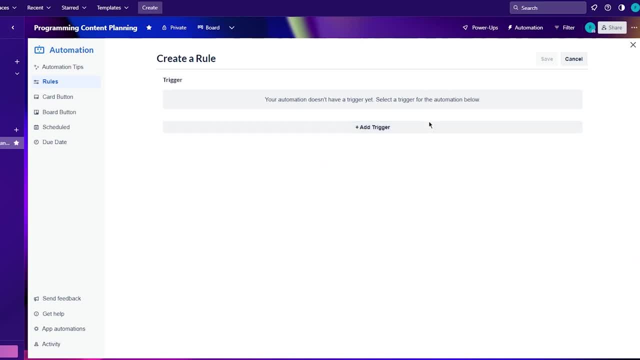 create. you are going to do that gear. obviously it's going to give you all the stuff. so first of all you're going to have to add a trigger. so once we can add a trigger, choose a trigger. so the trigger could be: card move, card changes, dates, checklists, card content fields and what you do that let's say. it states: 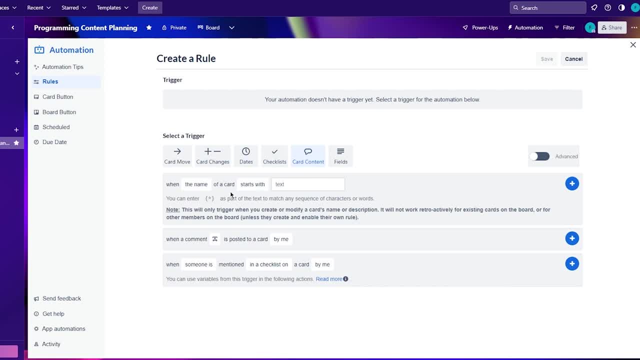 okay. or card contact with figures when a pre-registered decisions other than sairton, that ID or four plate numbers on top of this list. so once you said this, make all this. here I have a target option so when the name of a card starts with, you know, dash, you can enter this as a part of the text. 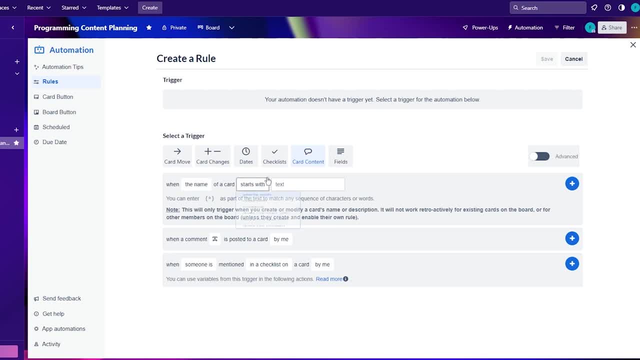 imagining sequence of the characters and once you choose this trigger, then you're going to basically add the action that is going to, you know, happen after this trigger. so you get the point. it's pretty, uh, easy and basic stuff to you know, get your head around like, not too complicated, not. 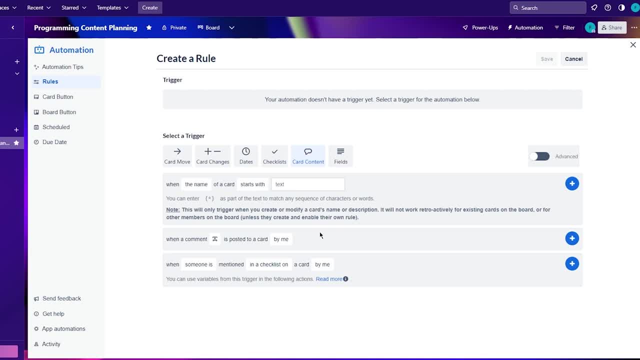 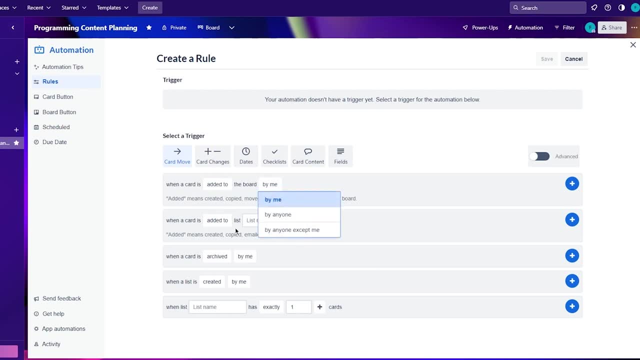 too difficult. so, as you can see, pretty simple. now let's go ahead with card move. so when a card added to board by me, okay. or when a card is added to the list name, choose any random list name- let's go development by me. when a card archived by me, when a list is created by me. you know all that. 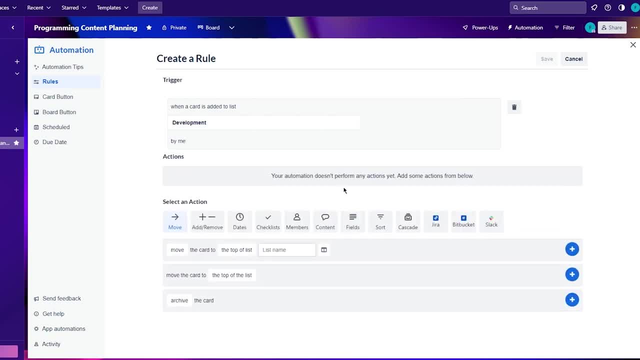 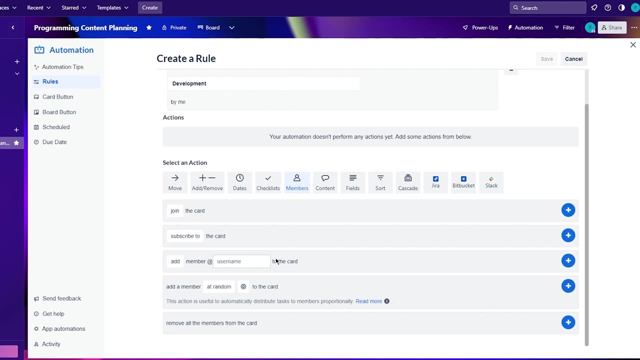 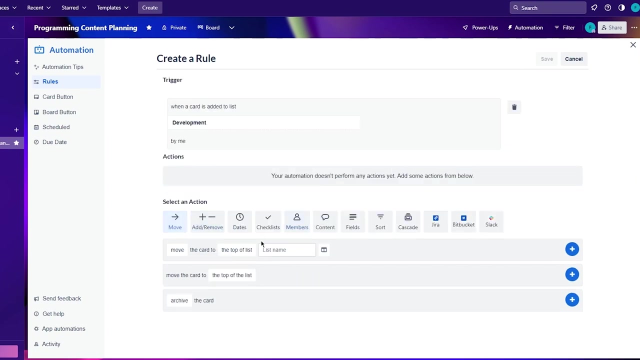 stuff. so i'm gonna go with this one. so that's my uh. you could say, uh, trigger. now the action that's gonna happen is, let's say, members. so you could say, uh, this, add member dash to that card. or, you know, add some other thing to the card depending on, or you can also keep this, so, when i like, add a card to the. 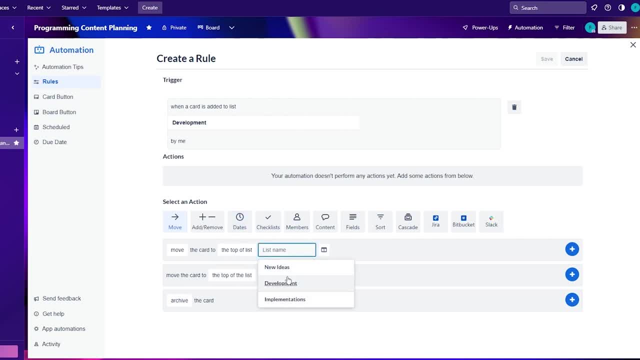 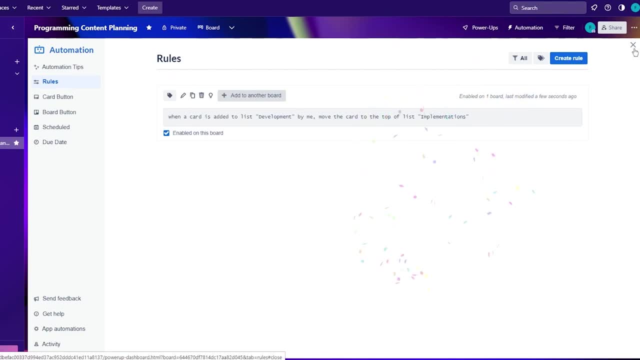 list development. move the card at the top of the list to implementation. so let's say i'm gonna go with this, i'm gonna click on saved and let's see what it does. okay, so i'm gonna come here. uh, first of all, yeah, let me show you the vote section. so this is voting. 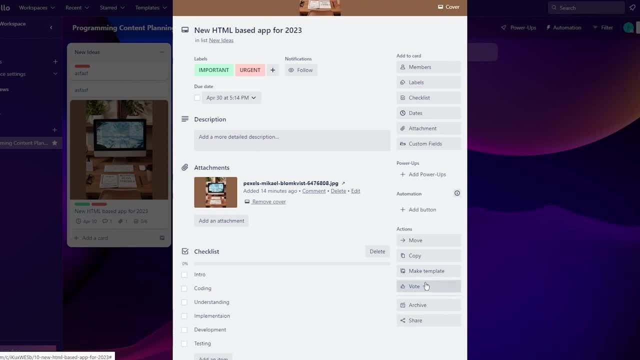 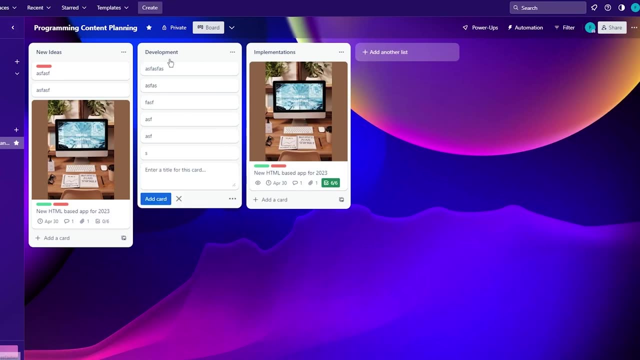 obviously this is the power up that i told you i would add. so that's the voting section, and again, mess around with it as much as you want. now, remember, i'm gonna add something and it's gonna add this into implementation. so look at that. i'm gonna click on enter and let's just 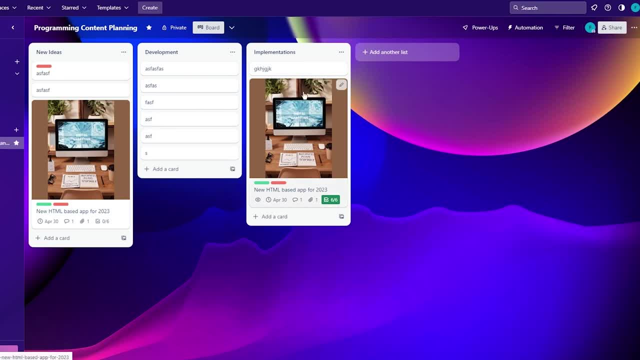 wait for it and look at that. it adds it immediately into implementations. how cool is that? and obviously i'm gonna add some more button automations in trello as well, and obviously they're extremely useful things to mess around with. so basically, to create a button automation for yourself. you. 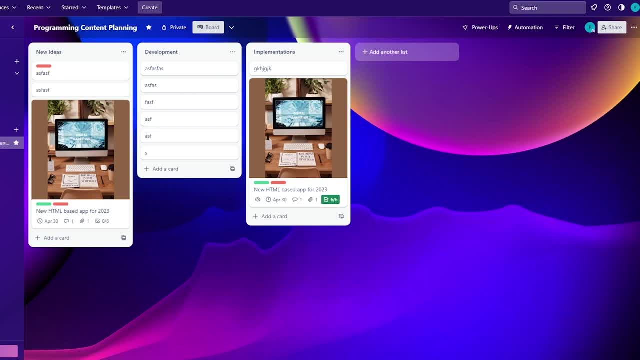 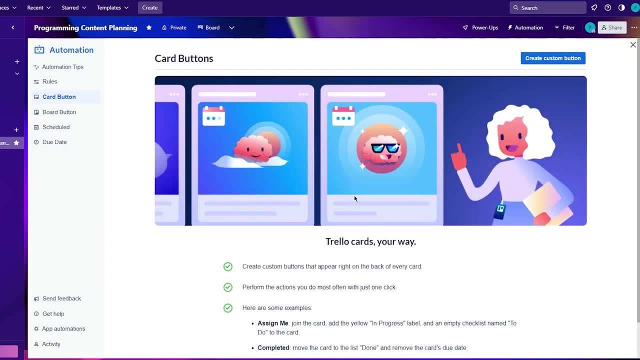 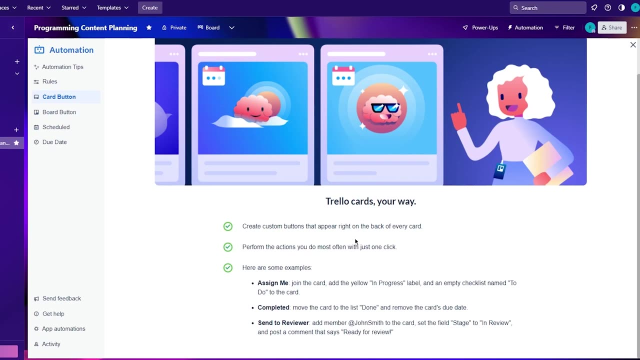 could just, you know, go in settings or you know, you could choose the butler and to choose that, obviously, go to automations, go on buttons over here and once you're in buttons, you can get this stuff accordingly. so, trello cards your way. create custom buttons that appear on the back of the 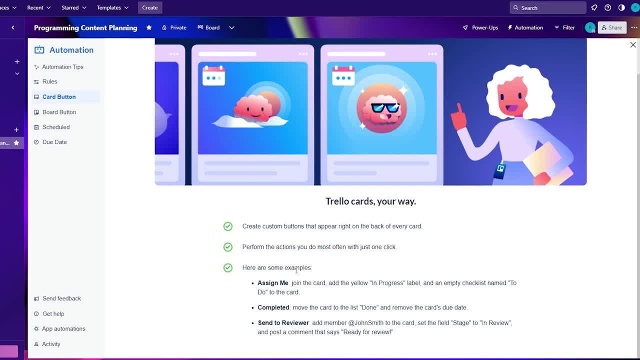 card so you can create custom buttons that appear on the back of every card, perform the actions you do most often with just one click. here are some examples. assign me: join the card, add the yellow in progress label and add an empty checklist name to do the card completed. move the card to the list. 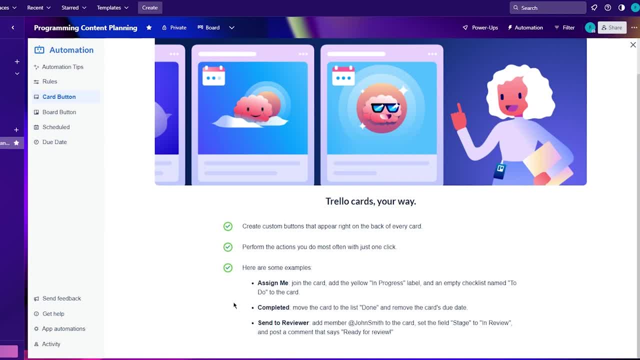 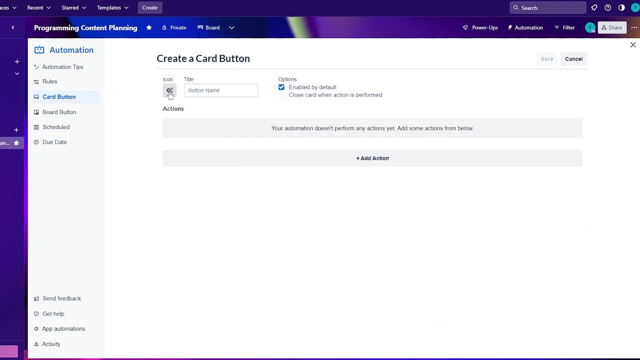 done and remove the card's due date, send to a reviewer, add member john smith to the card, set the field stage to in review and post a comment that says ready for review. so these are basically your card buttons. so i'm going to go and click on create custom button and here we are. so first of all, there's the icon. now in the icon, 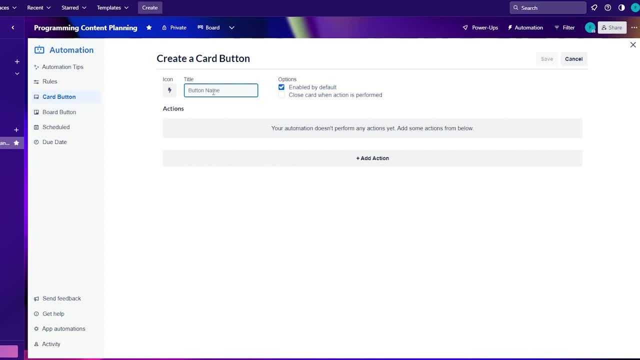 let's say i'm going to choose this lightning icon and i'm going to call the button name. let's say send to implement. i'm going to call it that you're going to choose enable by default if you want to. now let's go ahead and choose an action. so i'm going to choose on move top of the list to. 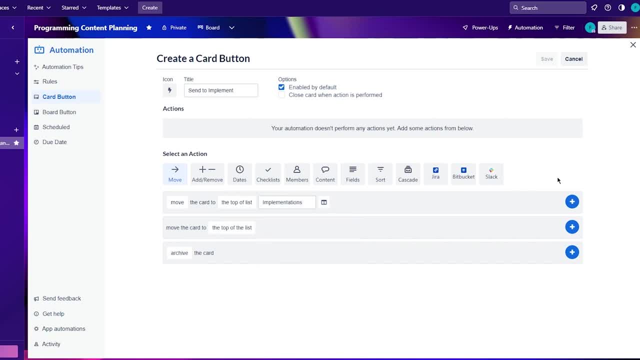 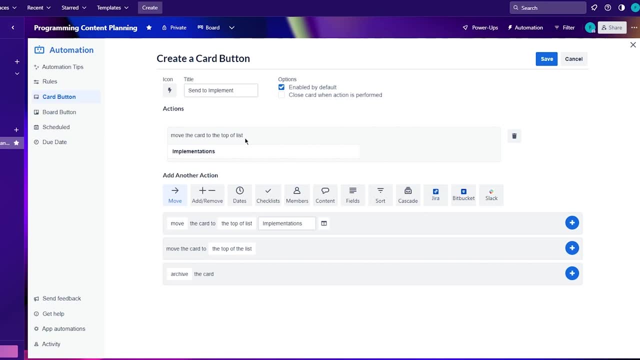 obviously implementation. that's our action and you know, just choose that. and once you choose that, you're basically going to be good to go. so, as you can see, moving the card to implementations and all that stuff, you can also do multiple stuff. so move the car to the top of the list if you want to. you know all that stuff. 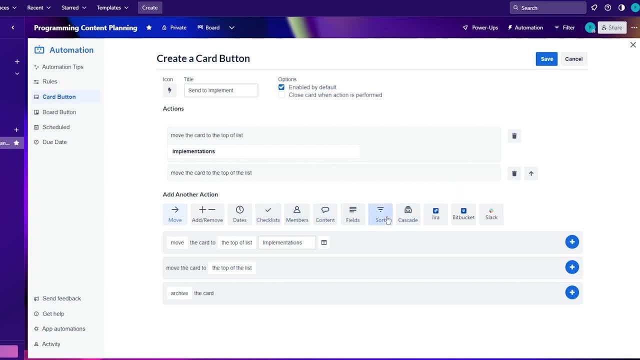 and you can choose different actions if you want to. from you know you also have gyra, uh, bitbucket, slack, dates, checklist, members content. you know all that stuff so you can accordingly add you know all that. so once you, you know have added all these actions accordingly, if you wanted to, you're going to. 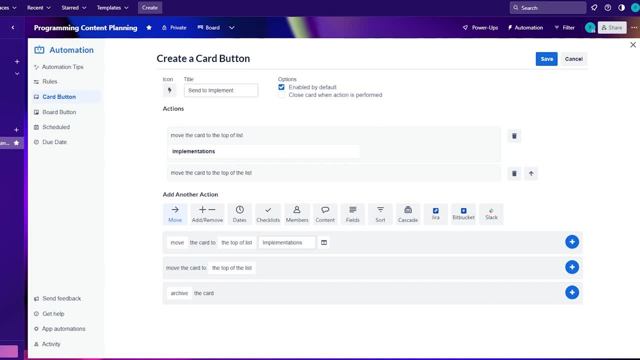 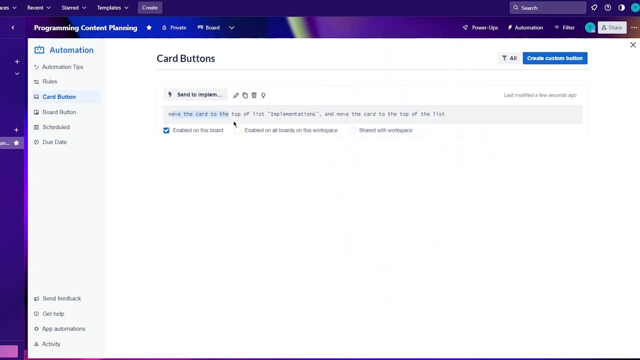 double check them. you're going to check that they work well with each other, because we don't want overloading, and once you do that, you're going to click on save so as you can see: send to implementation. move the car to the top of the list. implementation and move the car to the top list. 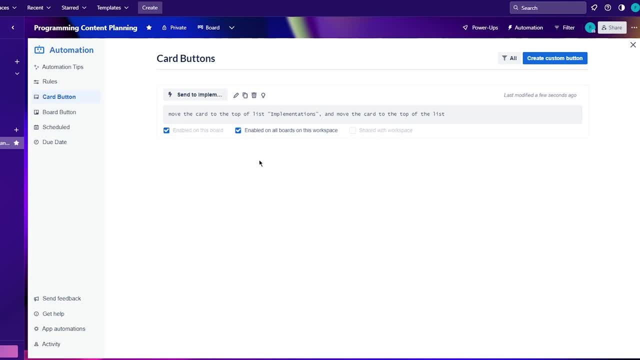 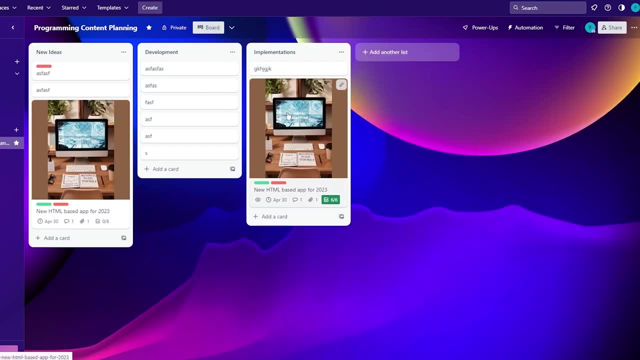 you know, once you do that, you can also choose this, which will enable this on all boards on this workspace. and once you do that, you can also choose this, which will enable this on all boards on this workspace. and once you do that, we're going to do this and, let's say, I am going to move this over. 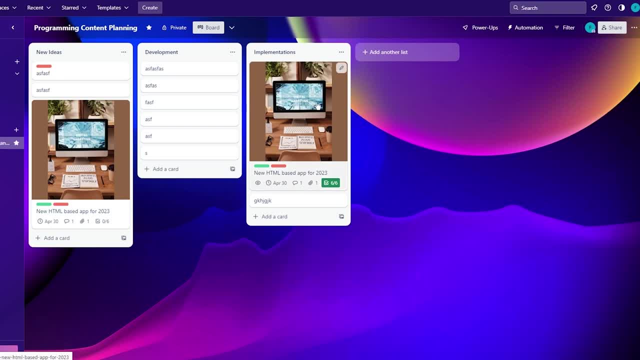 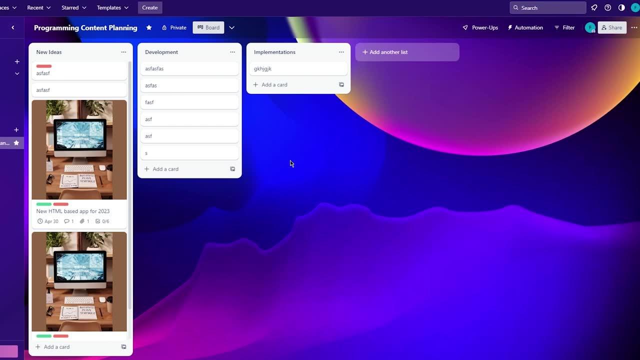 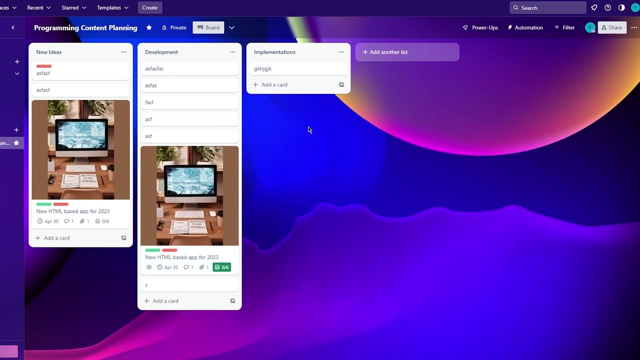 here, or maybe you know, move it, look at that. it's going to move it to implementation. so I'm going to move this over here and I'm just going to wait for it. so, like, obviously it doesn't move it to implementation and new ideas, but if you move it on development, just wait for it. look at that. back to 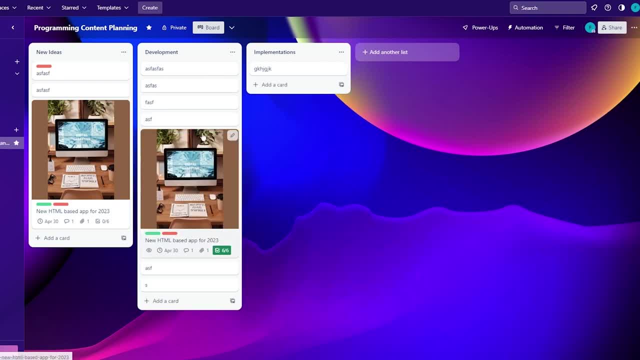 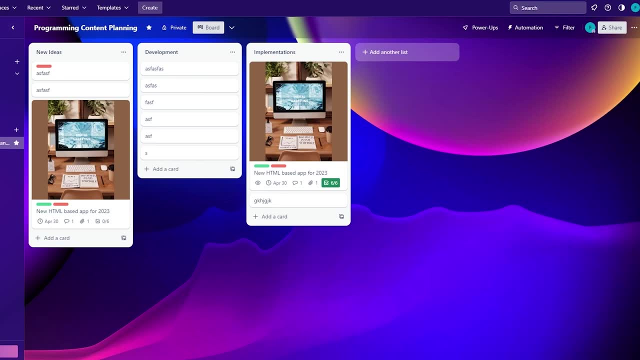 implementation. so you can't move anything out of implementation. it's obviously eventually just going to move it back to implementation from development. now, once that is done, let's go ahead. and obviously I discussed the importance of filters in the start of the video, but again, filters are one of the most necessary and important things when it comes to Trello. 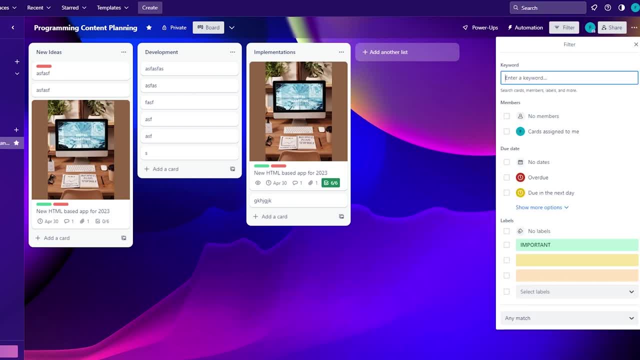 because they allow you to basically have a much easier look towards these new faces. so you can move this over here and you can see that it's moving this forward. so you can move this forward, so you can move this to implementation and then you can move it backö. 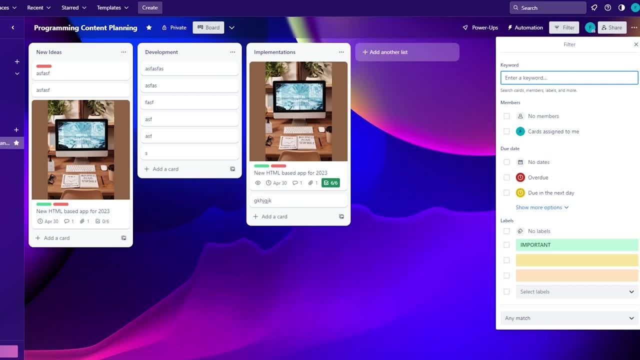 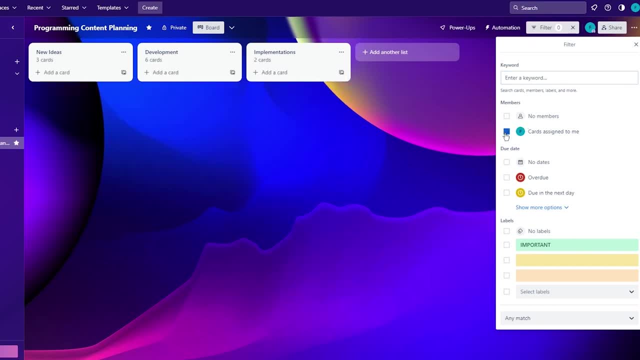 the board because they help you get around the board pretty easily. so if you were to click f on your board, you see it's a pretty good, quick shortcut and, as you can see, you can choose the cards assigned to you, choose it for no members, you can also choose the due date. so let's say, 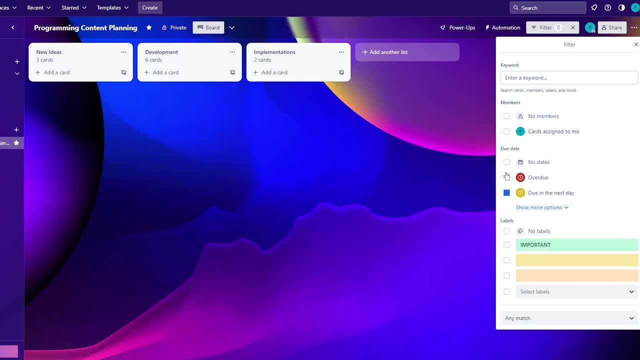 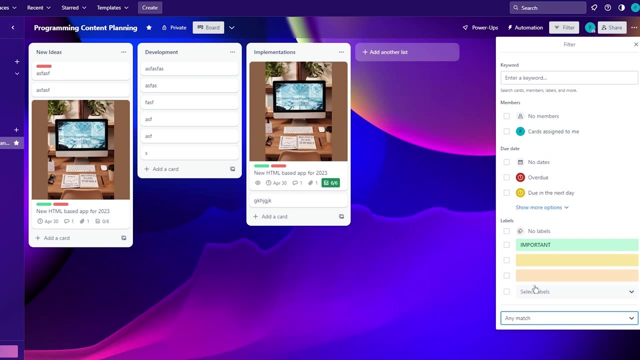 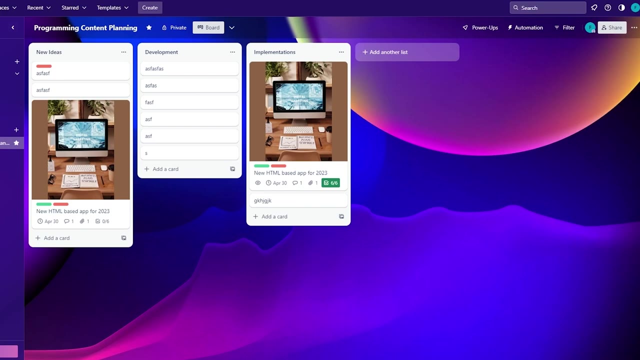 this due date is, you know, overdue, due in the next day. all that stuff, choose the labels that you want to go with exact match if there is any, you know, all that stuff. so again, pretty useful thing to have in your board and it's a good thing to just, you know, know how to use, to be just pretty. 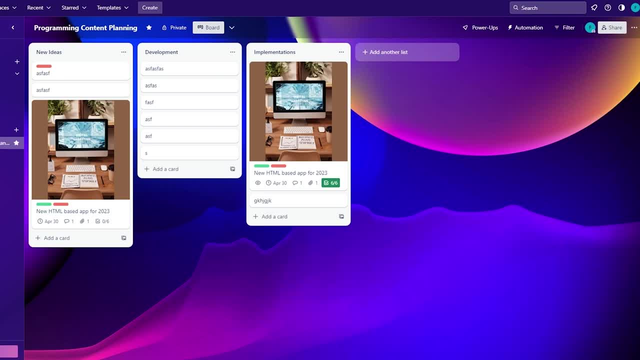 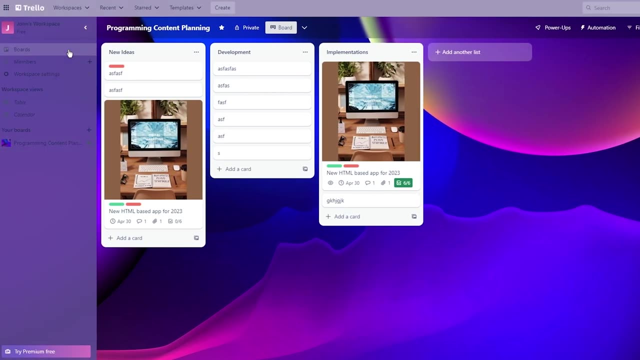 familiar with, familiarize yourself with all these features that i showed you and, yeah, you're going to be good to go now. this is obviously for your work management. you can also create a board for, let's say, like for your personal boards. okay, so let's say i'm going to go on boards over here. 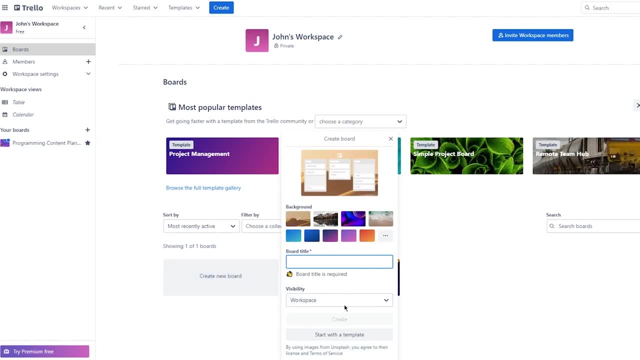 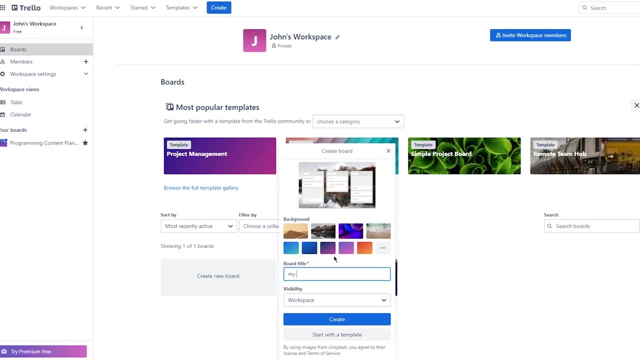 and i'm going to create a new board for myself. so let's say, i'm going to create a new board and i'm going to choose, like a random background and i'm going to call this, uh, my goals. i'm going to call this board my goals and once you do that, you're going to click on create and once you click, 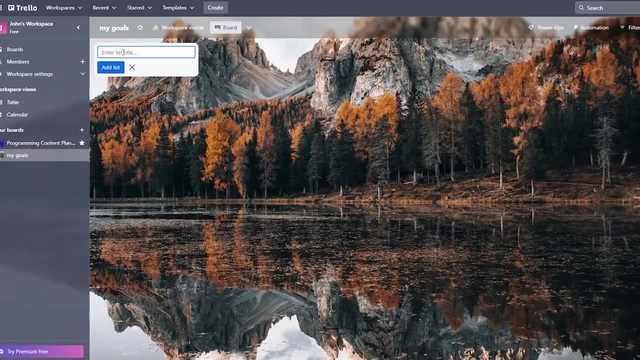 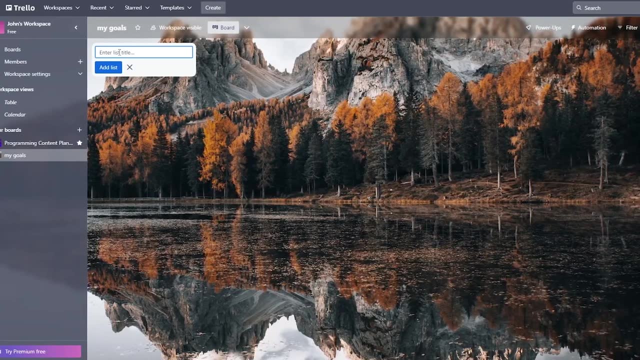 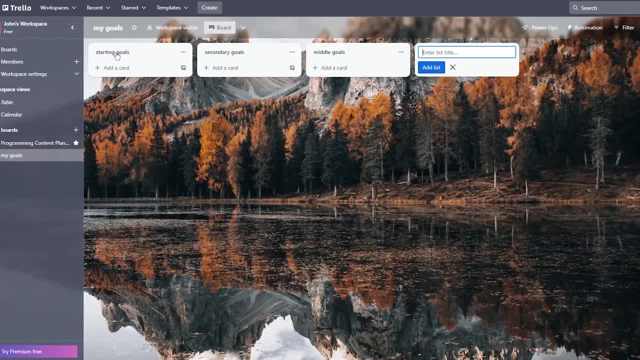 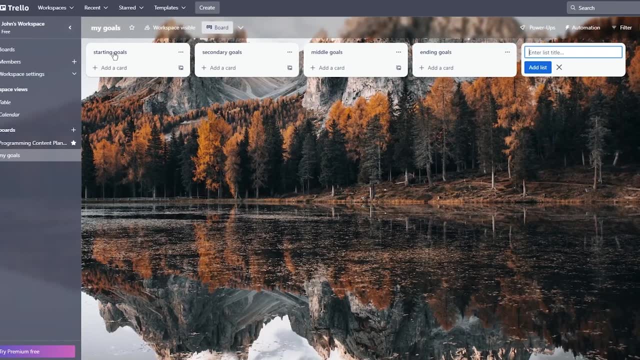 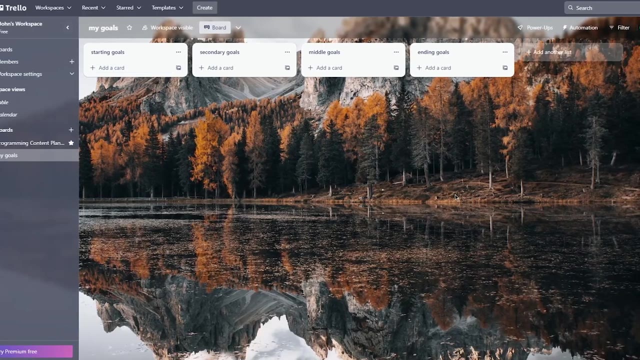 goals, middle goals, and you know accordingly, just choose as many and then ending goals and all that stuff, and obviously over here you can add in your goals accordingly. you can also choose days for different. you know goals that you want to add and obviously this is for your. 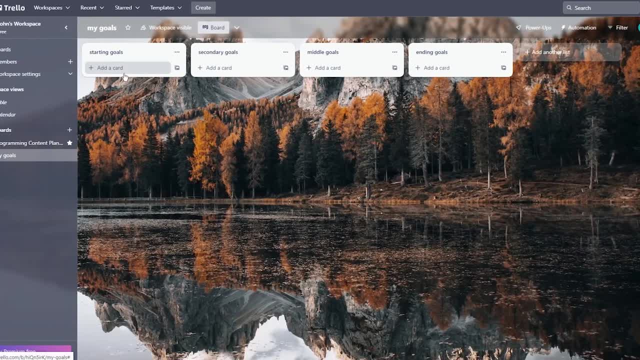 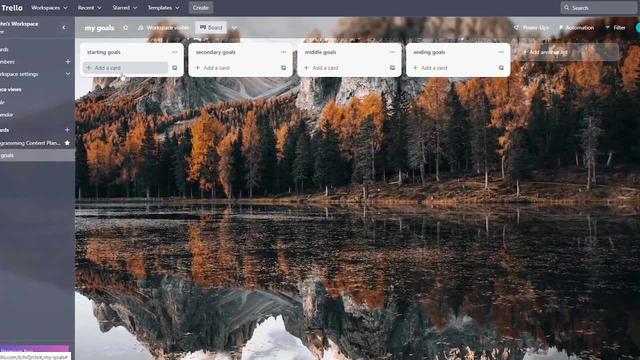 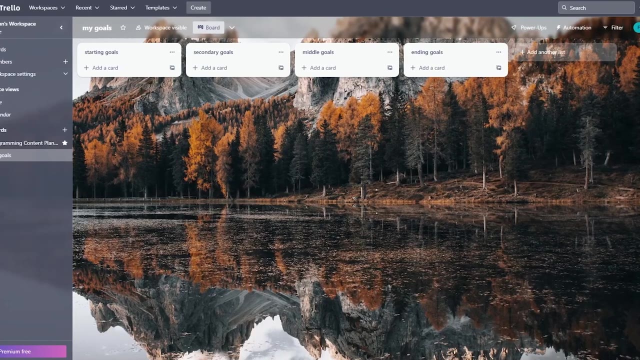 personal stuff. so in over here you can add a card for you know. uh, let's say, starting goals could be doing gym, doing exercise, losing weight, starting the diet, and you could add different back burners if you want to, or it could be, you know, maybe you're. 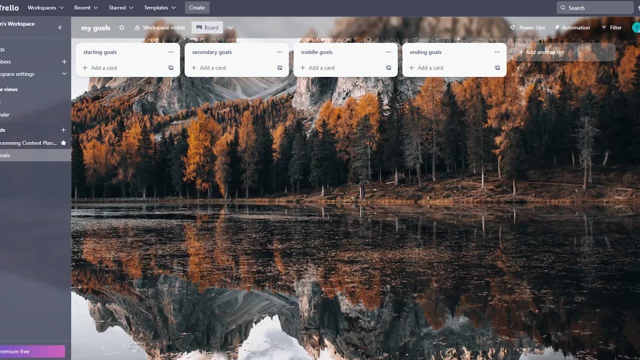 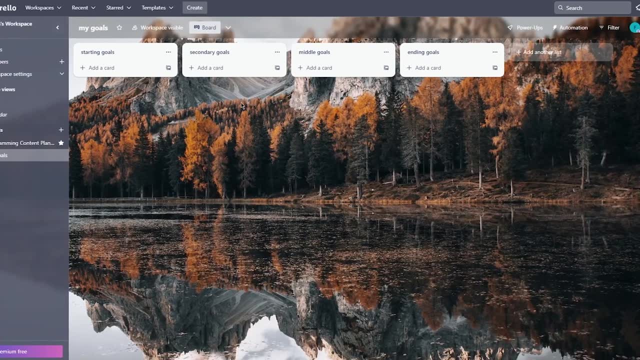 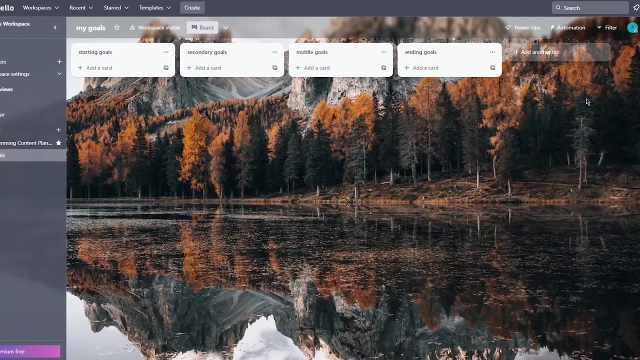 writing a book and you want to complete that. you know all that stuff again, a lot of things that you can, you know, get behind, and all that stuff- and this is basically your goals- that you can mess around with. you can also use trello to plan your day, if you want to. okay, so to use trello to plan. 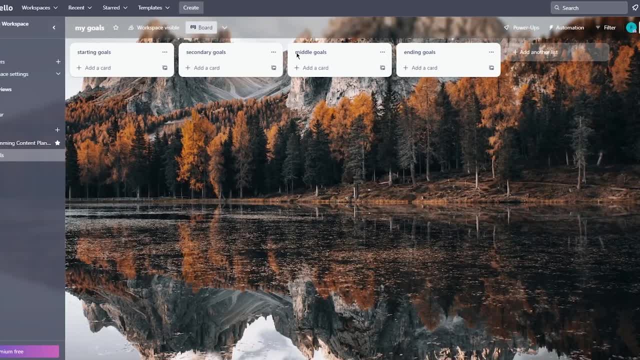 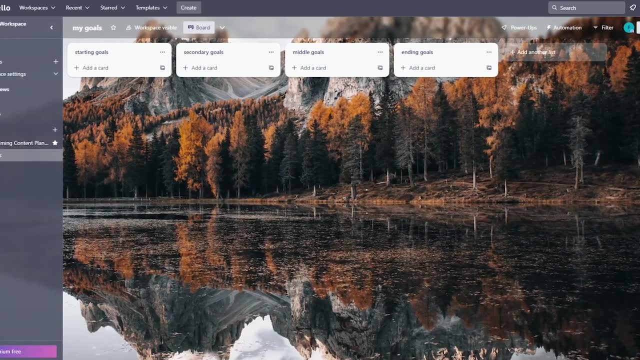 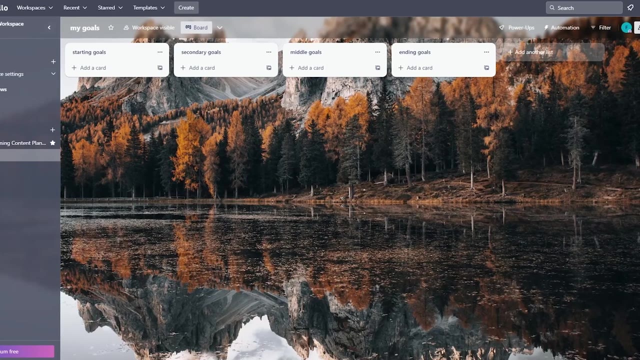 your day. basically again same thing. just choose monday, tuesday, wednesday, thursday, friday and then make a single card for the weekend and then accordingly put in tasks if you want to. and once you put in tasks, keep you know times for that task. so let's say on monday, or like let's say on: 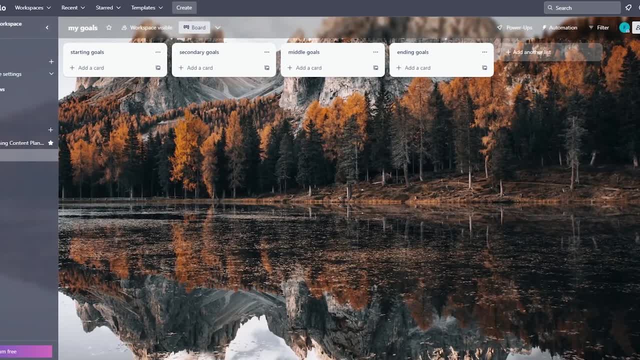 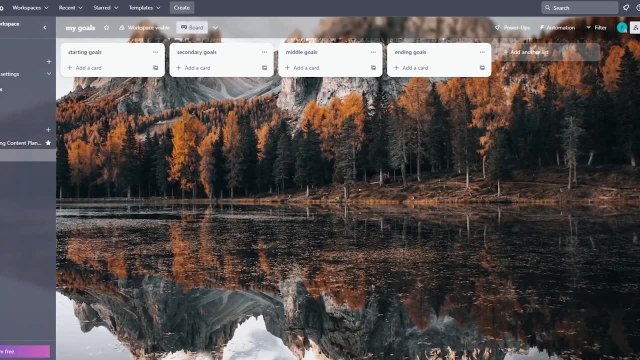 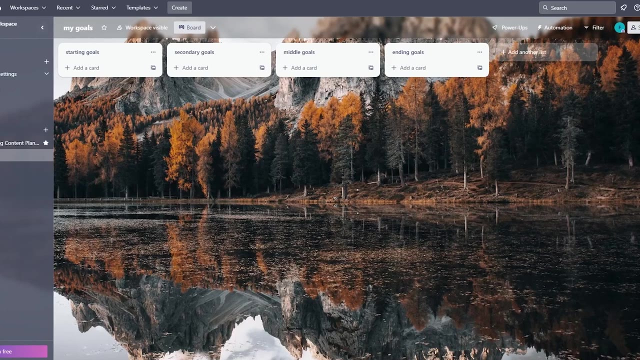 the morning morning routine, we're supposed to drink half a gallon of water, eat breakfast, shower, work out and once we have done all that, then comes, you know, task two in the monday routine. on monday, you know, change of clothes, put on cologne, you know, look good and professional, go for work. then obviously, talk to your boss about some you. 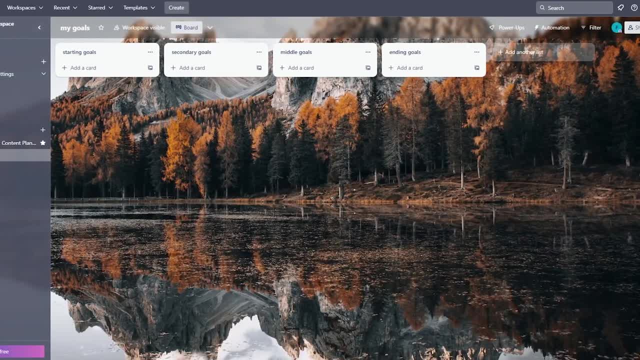 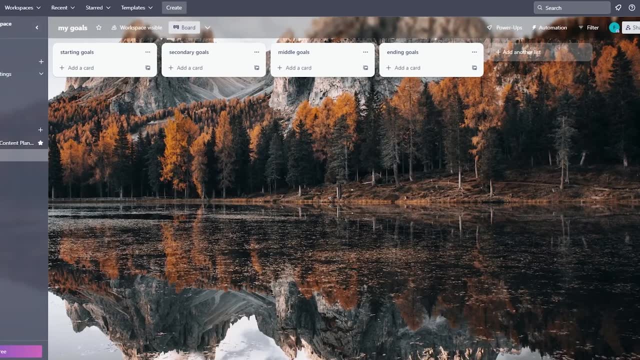 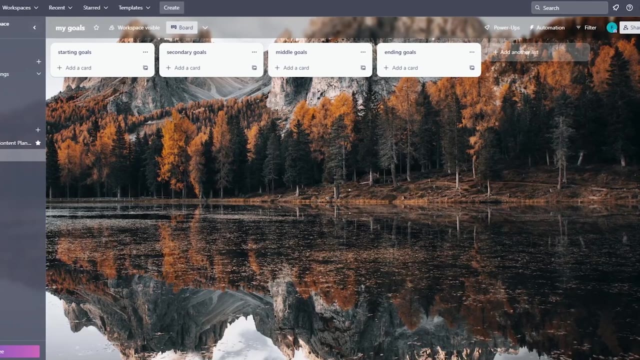 know important thing, for example. so, basically, you're going to set these tasks for yourself, just so you can, you know, make your life easier for yourself. and trello. trello is one of those softwares that you can use to just have ease of use, and you can, like use trello a as a proper 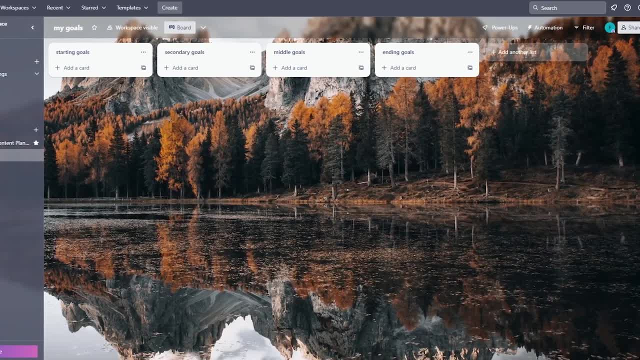 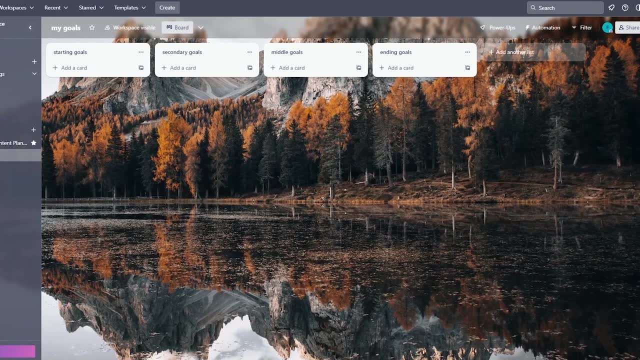 roadmap for yourself, if you don't know what roadmap is basically. uh, a whole map of your journey that you're gonna be doing in, like you know, a certain time period. so that is a proper roadmap and again, you can use that as a roadmap. uh, it could be. you know a software. 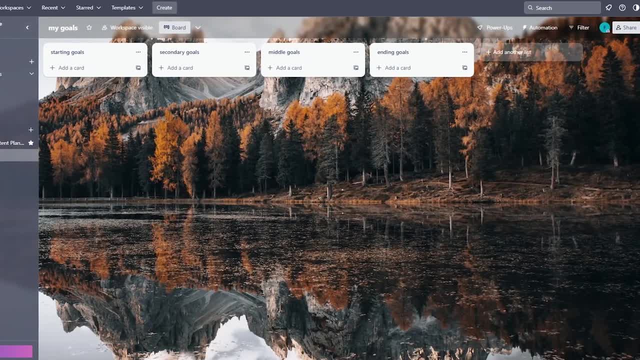 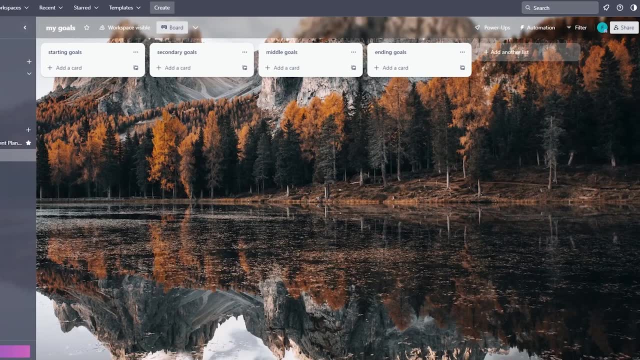 service roadmap. you know, hardware service, it could be any type of service roadmap. it could be a roadmap for yourself, maybe your mental health, physical health, all that stuff. so yeah, and once you've, you know, done a roadmap for yourself. uh, also, there's the map view. okay, now 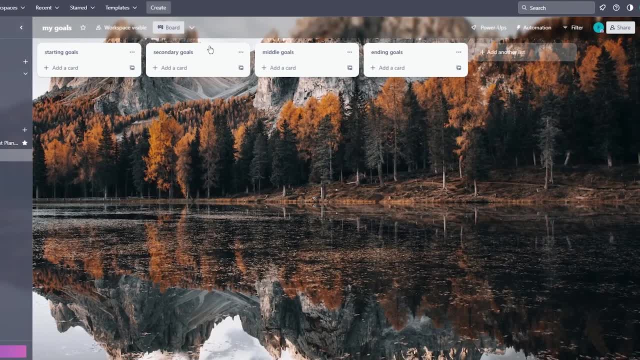 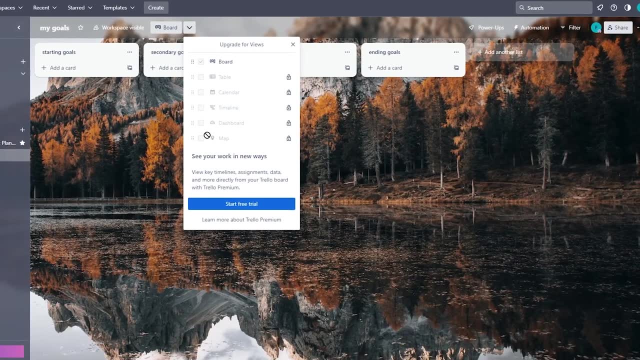 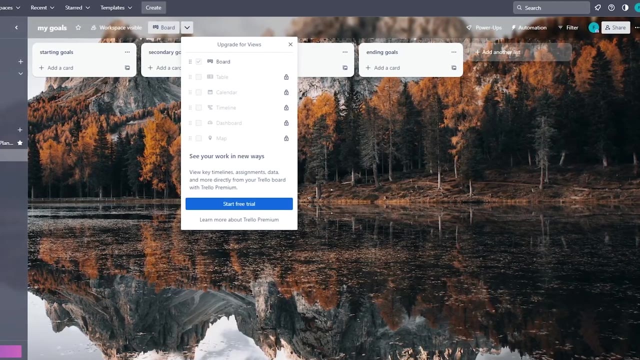 the map view basically comes in like, obviously in like the different views. so you're gonna come to board and over here you have map view. obviously, again, we can't use it because we're not on like the premium plan. but once you're in the premium plan, you should use and check out the map view, because 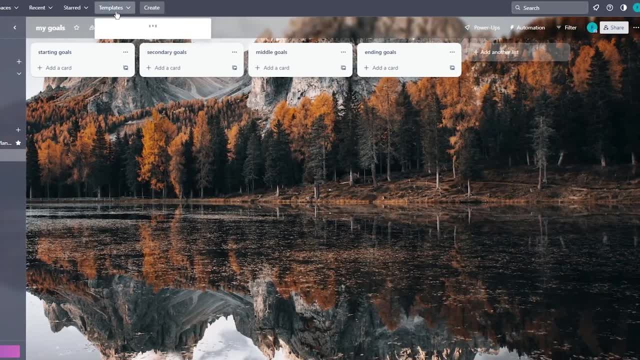 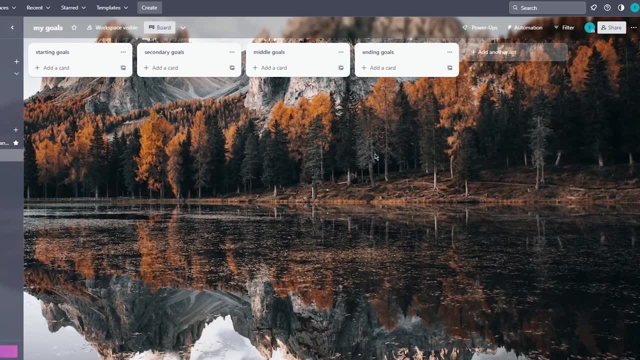 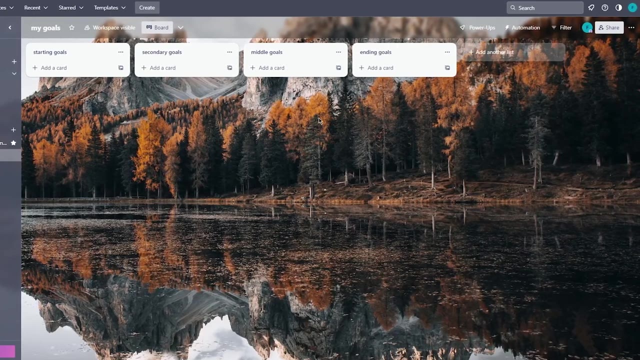 it's pretty useful when it comes to working with trello and it gives you a great look on how things actually are. it's going to give you a whole map view of like where your work consists and all that. so that's pretty useful and i recommend that you use it as well. then, obviously, there's the timeline.